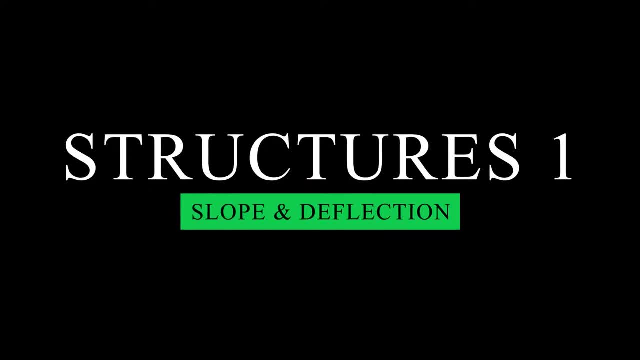 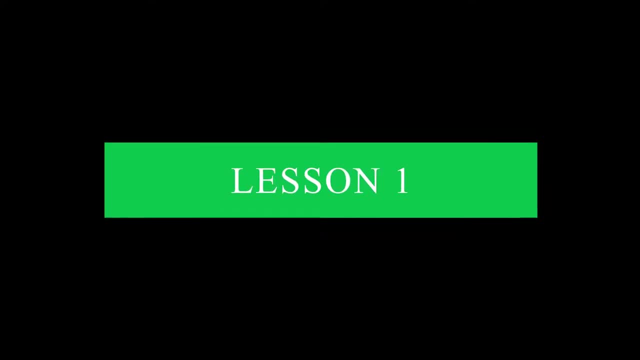 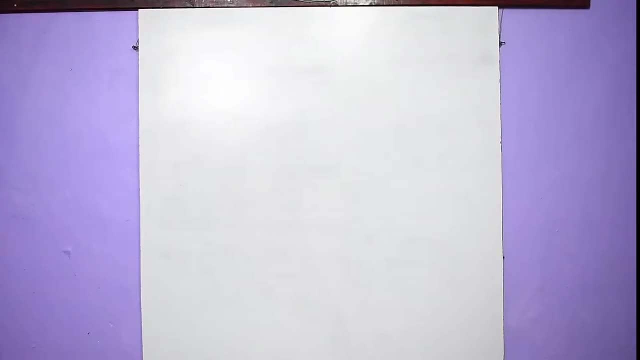 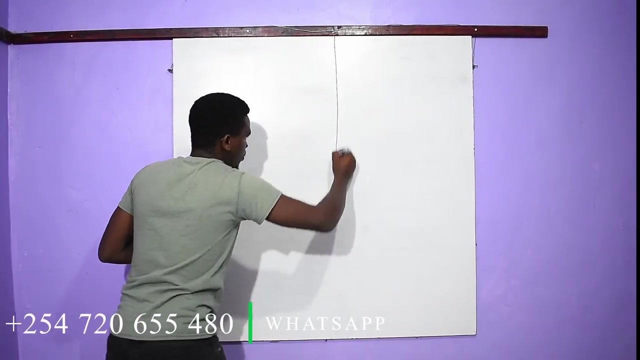 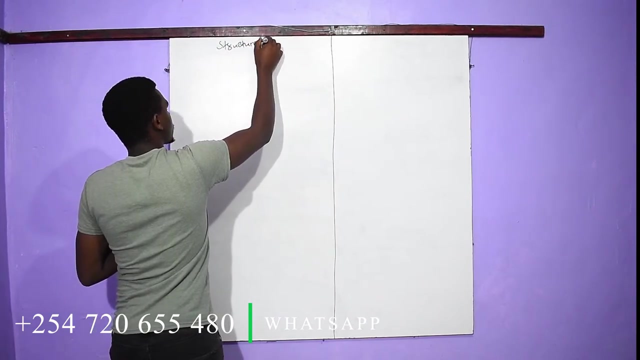 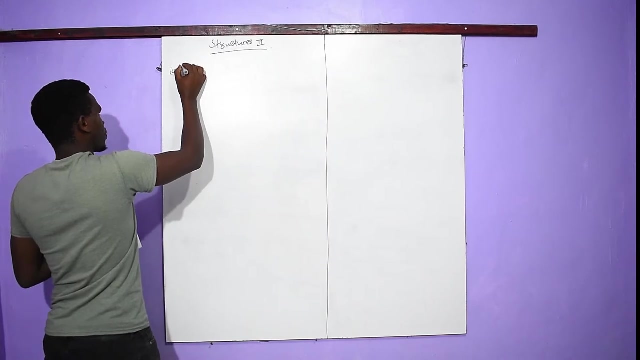 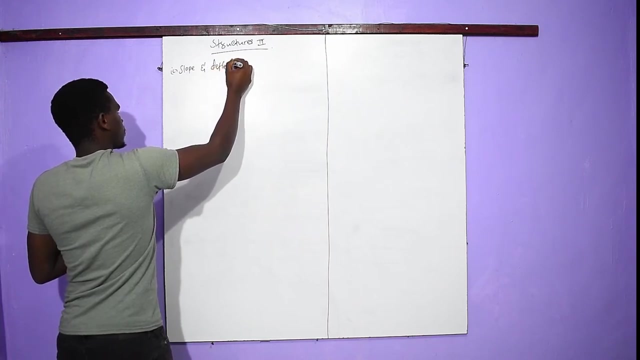 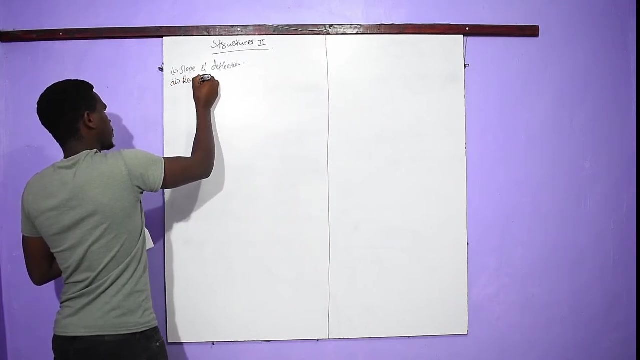 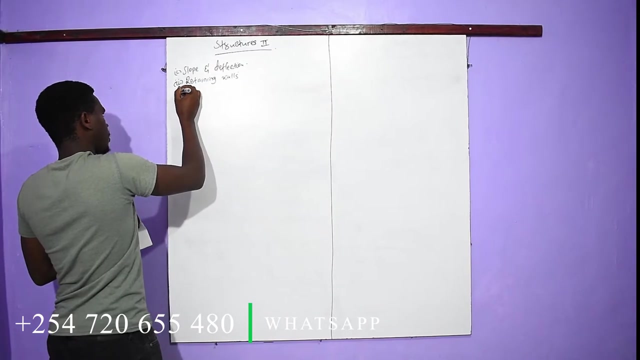 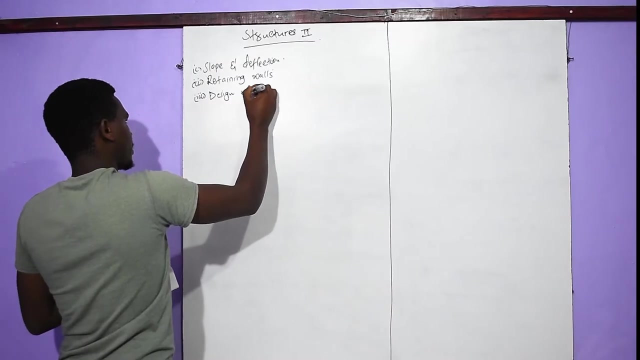 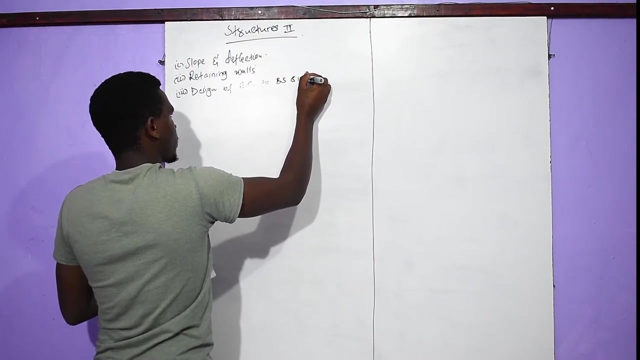 So today we are going to have structures, Structures, structures 2.. In structures 2, we have three topics: One is slope and refraction, Two is retaining walls And three we have design of reinforced concrete to BS8110.. So for today we will have slope and refraction and retaining walls. 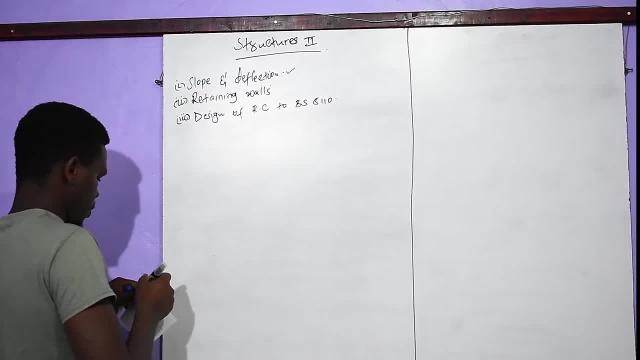 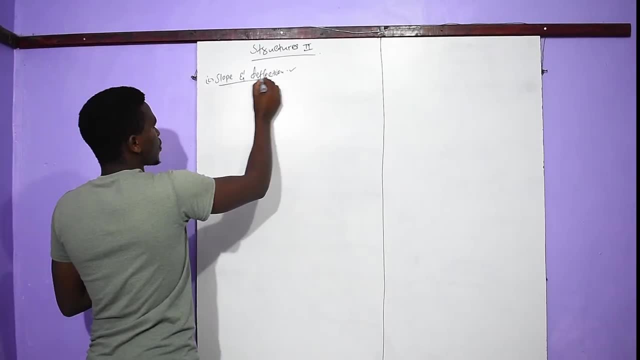 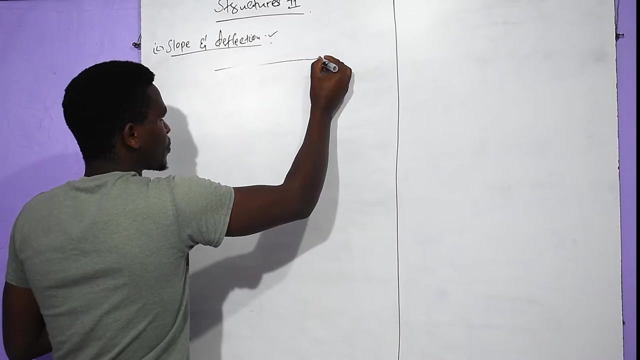 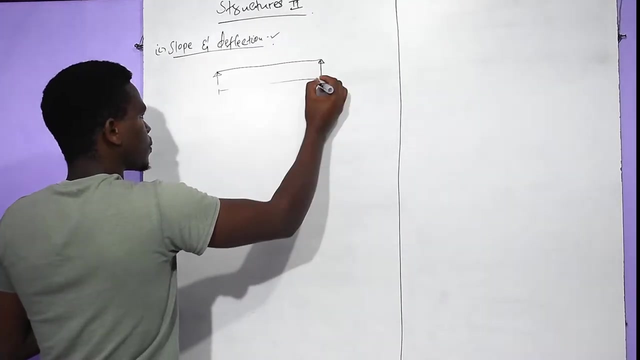 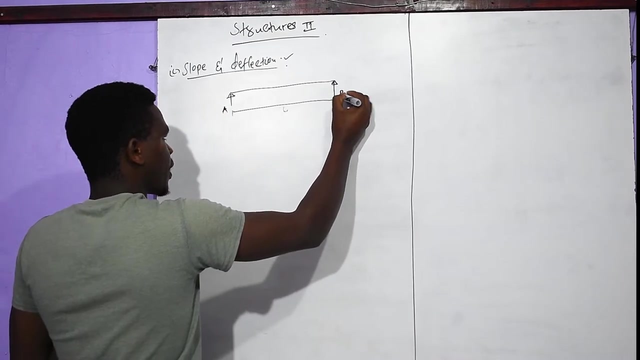 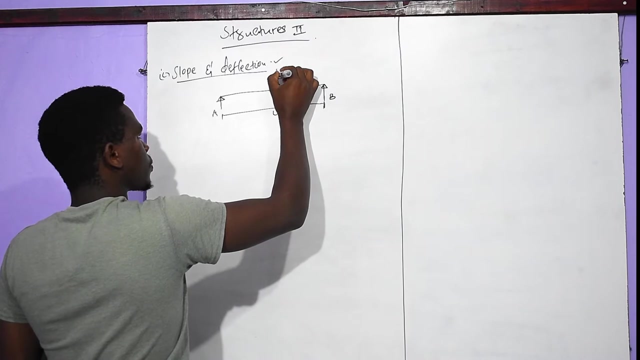 Design of reinforced concrete to BS8110 will be discussed at a later date. Thank you, So you have slope and refraction. Okay. So you take a piece of a simply supported beam with a span L, support A and B, put it at the center. 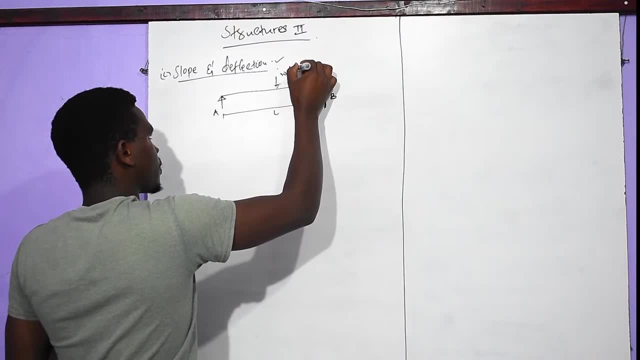 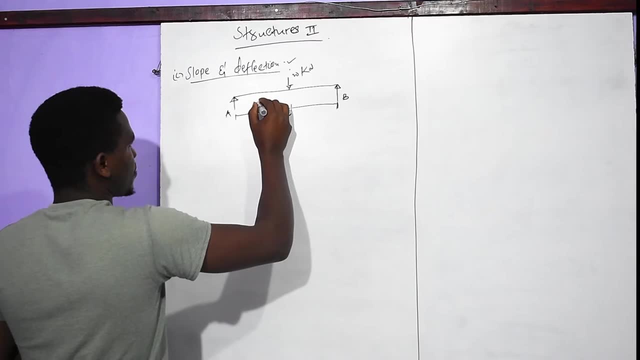 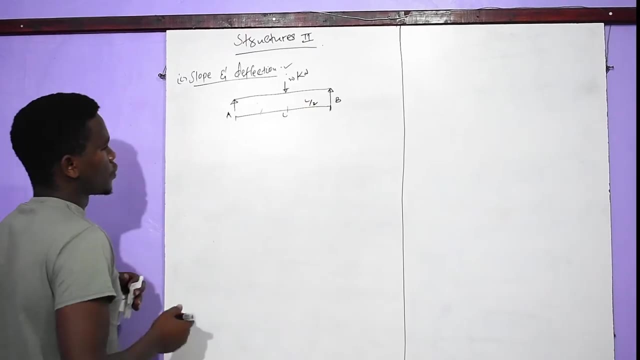 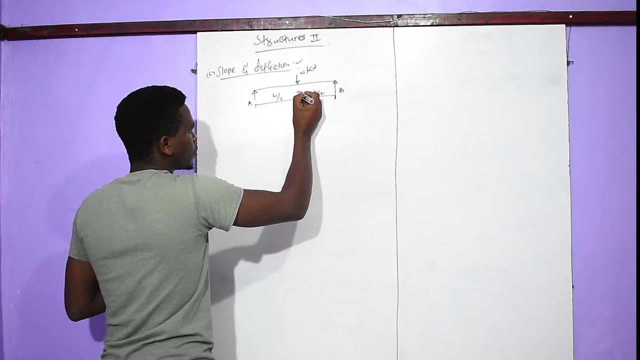 with a load Wk, kilonewtons Like so. So it is acting at the midsum, So this one is L over 2.. And this is L over 2. So when this beam is loaded it tends to bend. 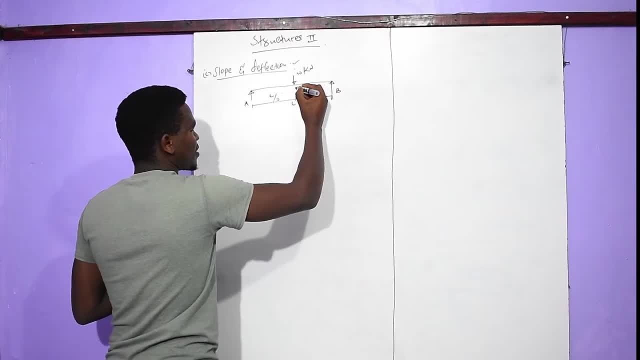 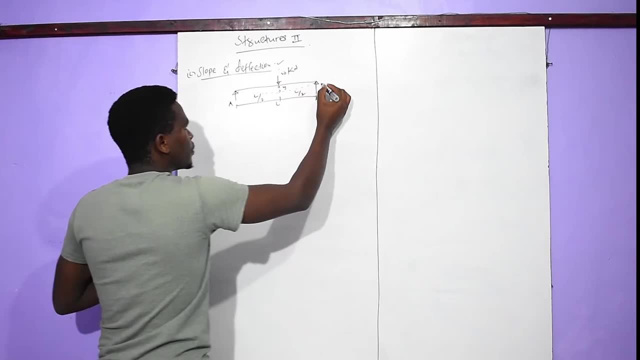 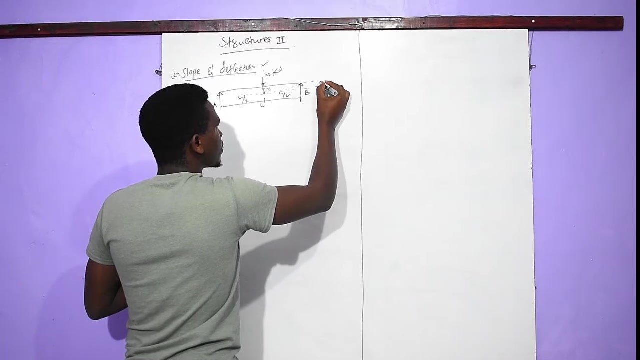 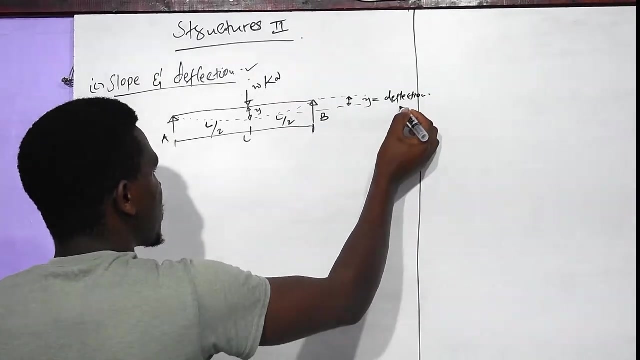 Like so. So when it decides there is this maximum sagging here denoted by Y, And this distance- Y is what we are referring to as refraction- This means that the beam deflates. So when we have the slope here, when a tangent is drawn to this curve, 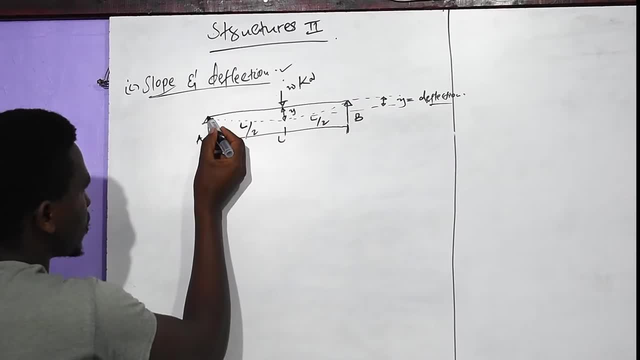 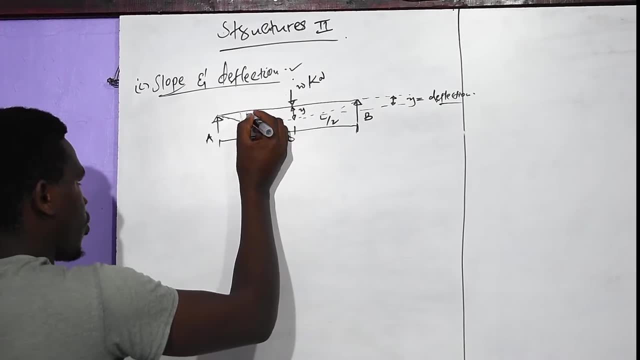 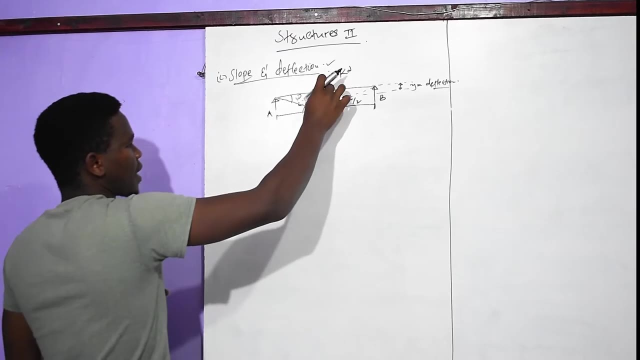 because this one will tend to be a curve. it makes an angle with the horizontal axis of angle theta Like so. So this angle theta is what we are referring to as the slope. Well, this distance from the horizontal axis, the maximum bending of the beam, is what we are referring to as the deflection. 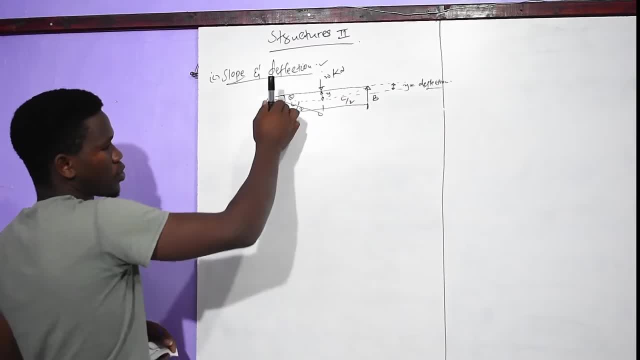 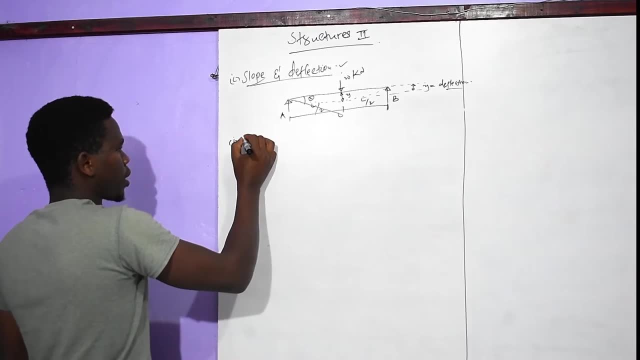 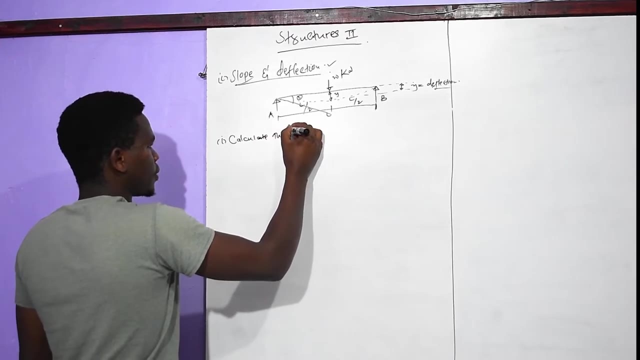 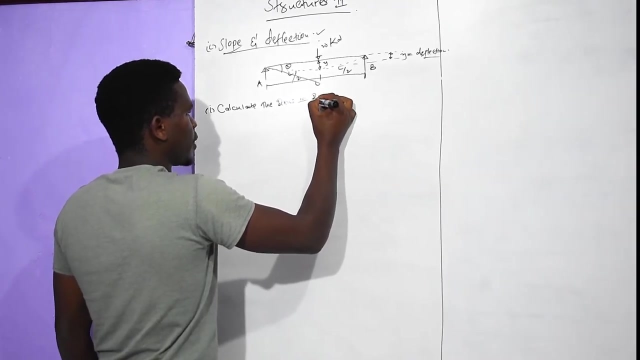 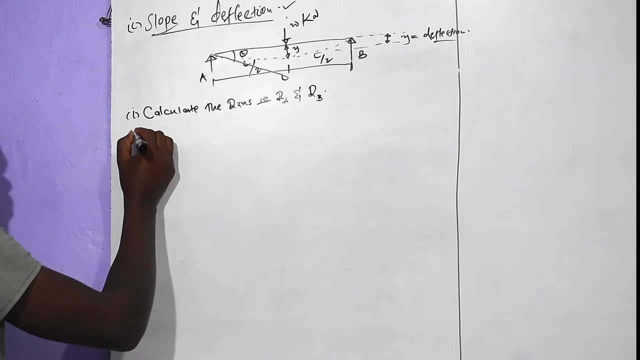 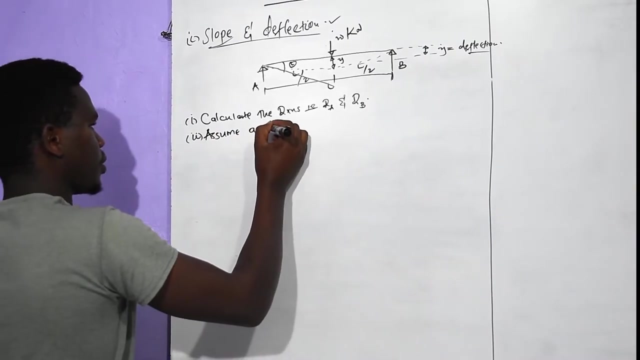 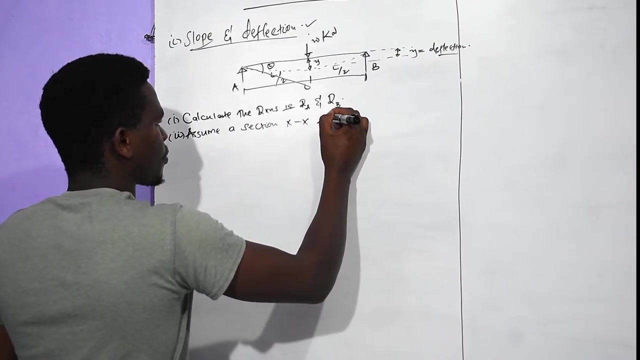 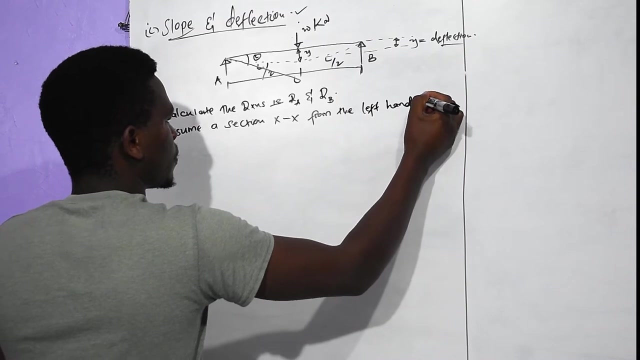 So for us to calculate the maximum slope and the maximum deflection, some steps are followed. Step number one: Calculate the reactions, That is, reaction A and reaction B, Like so. Number two: You assume a section a, section XX, from the left-hand support. 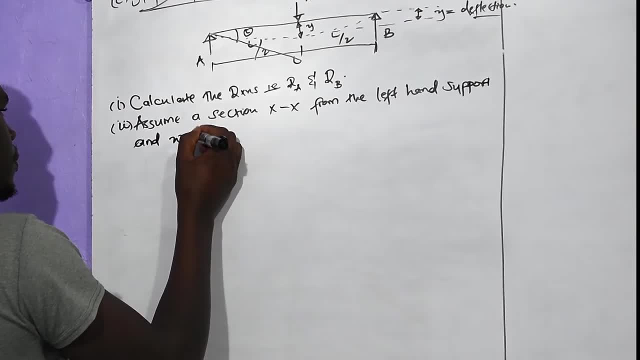 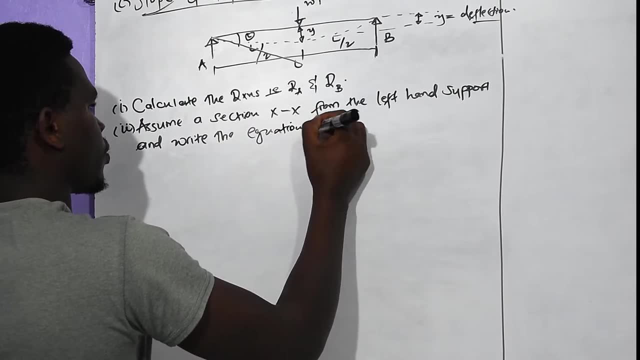 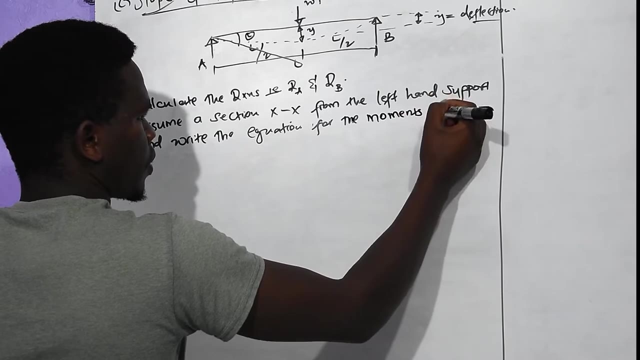 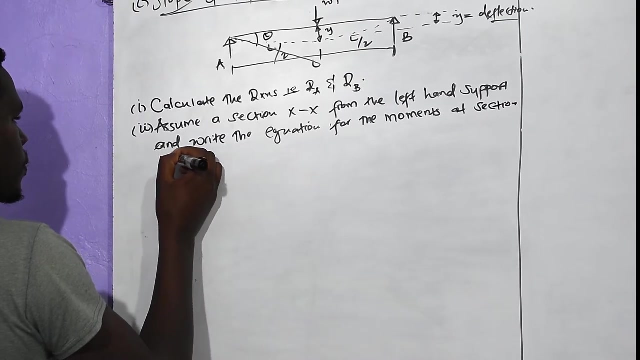 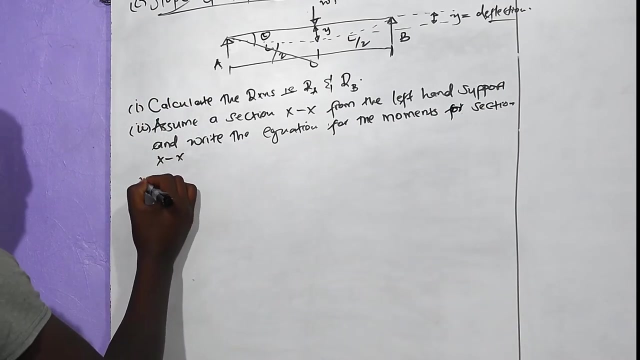 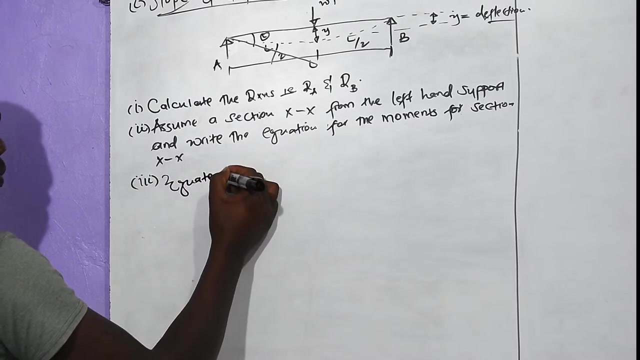 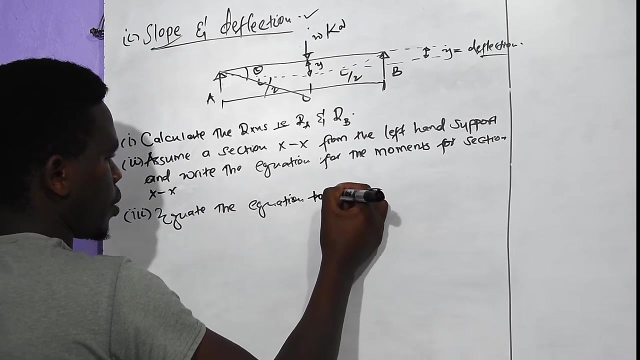 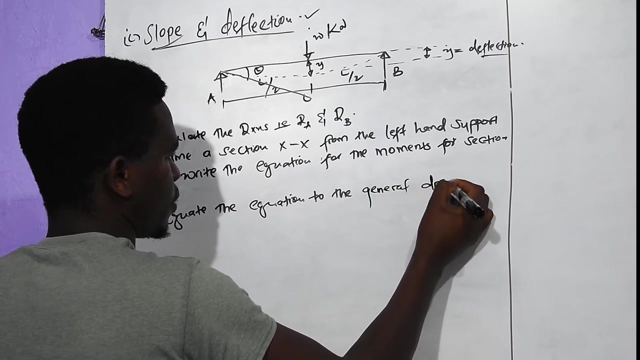 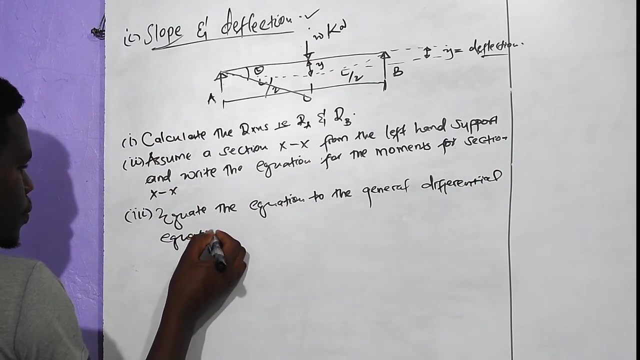 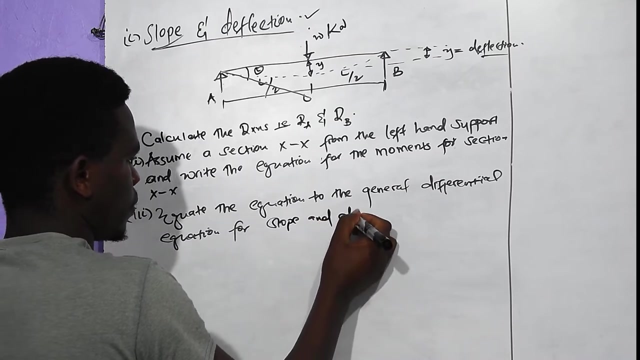 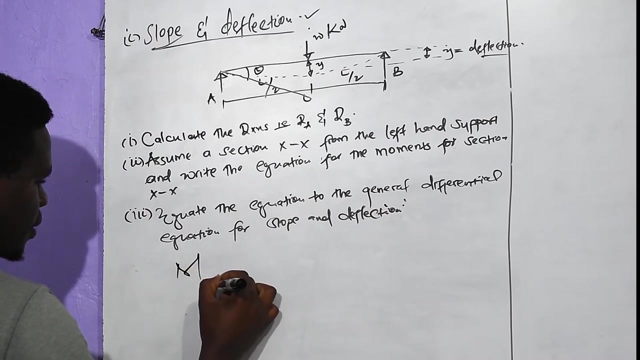 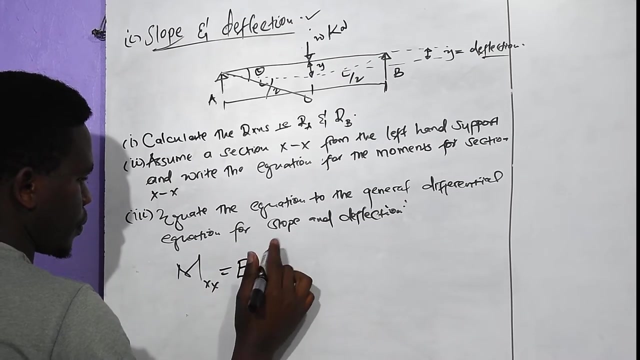 and write the equation for the moment at section XX. Like so, Number three, You equate The equation, The general differential equation For slope and deflection. Like so: Therefore, the moment XX will be equal to E. I. 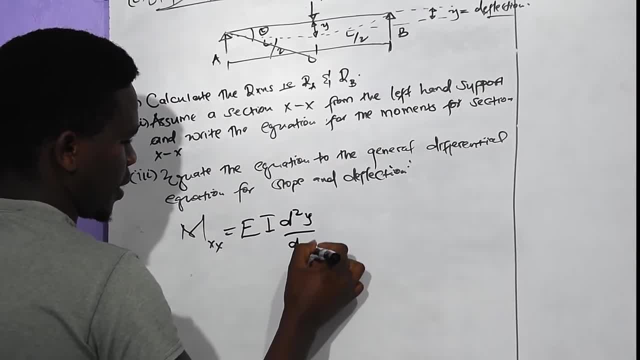 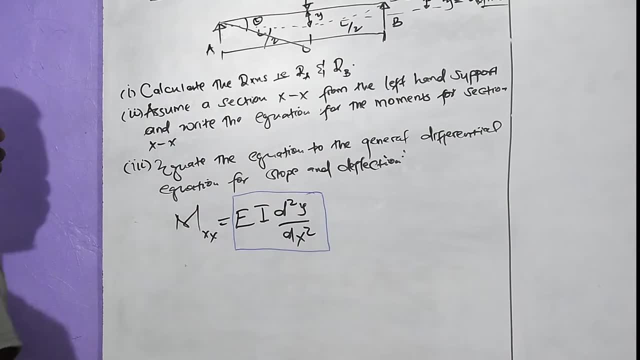 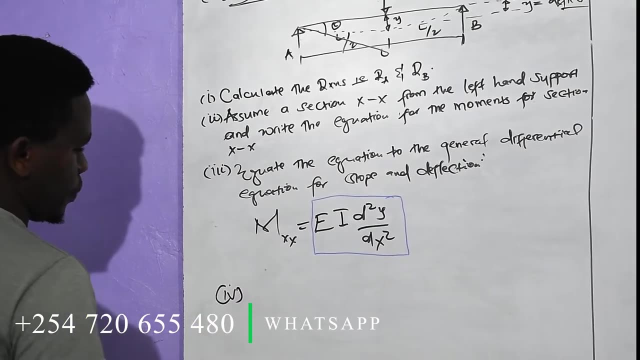 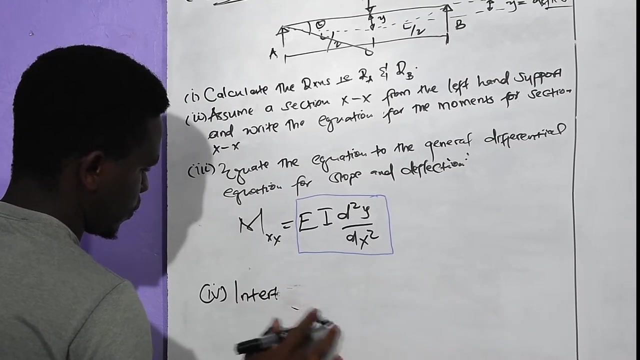 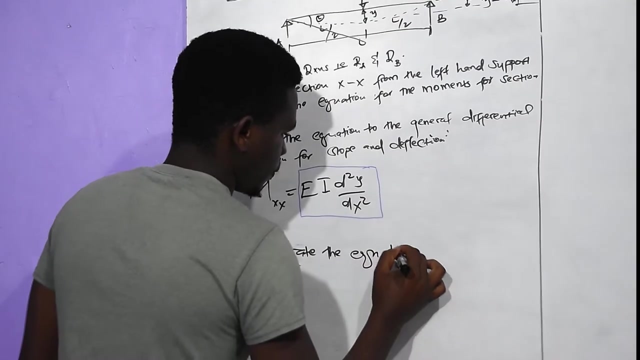 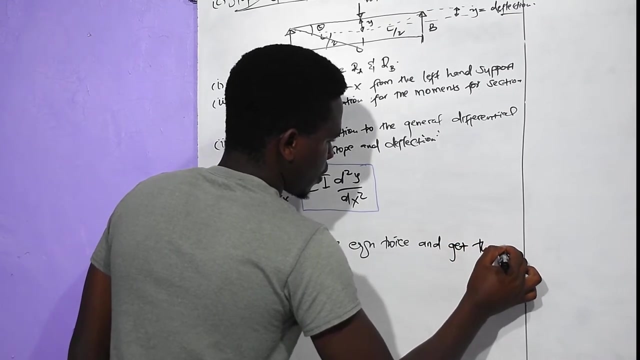 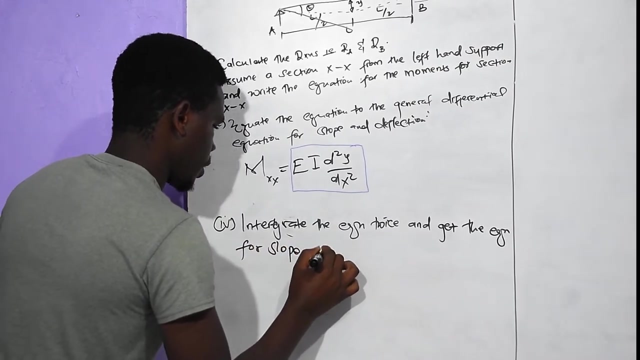 D squared, Y over D squared. This is the general equation, Like so For general differential, the equation of slope and deflection. Number four: Integrate The equation twice And get The equation For slope and the equation For deflection. 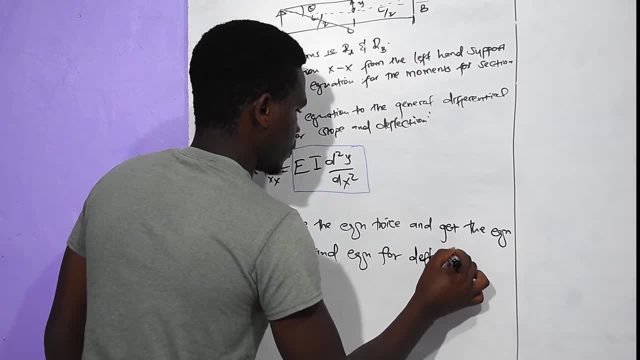 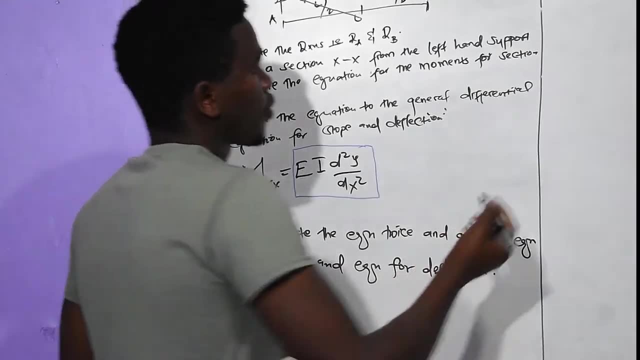 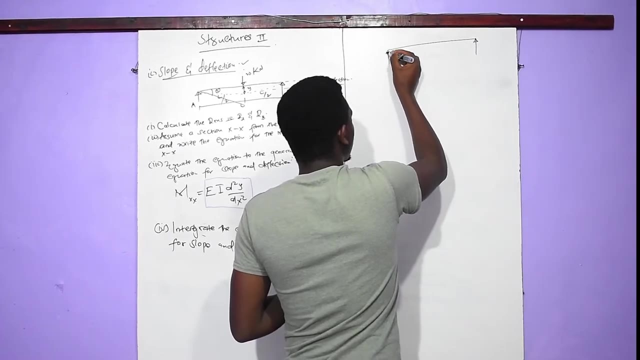 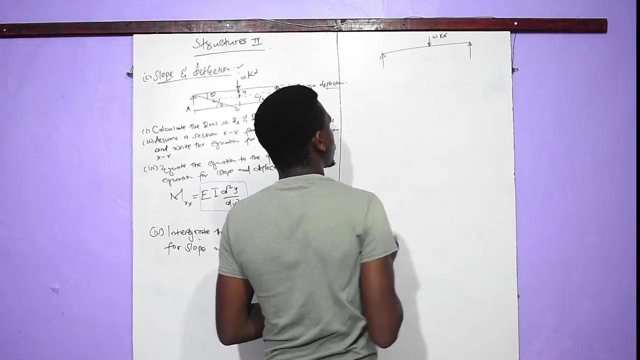 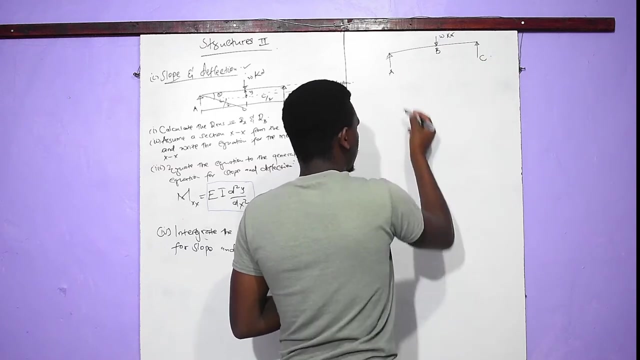 Like so. So for a beam, for a simply supported beam, Like so: And this is the Interval of the beam, The angle of the beam. Here you can see That there is This A line And this is the. 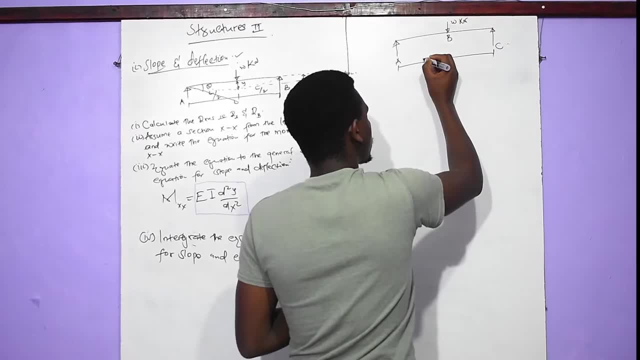 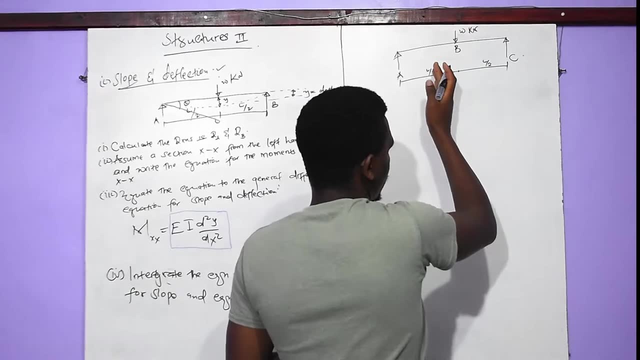 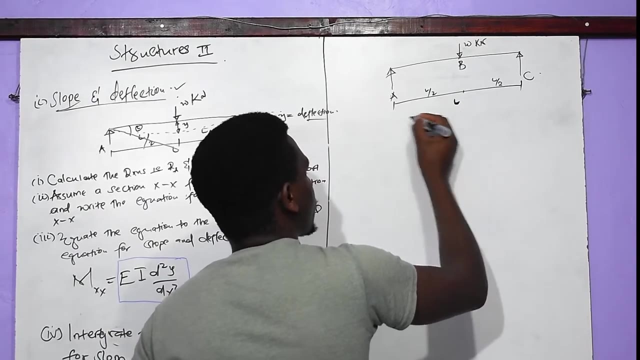 The angle of the beam. Not as long, But this is the The, since it is acting on the mid-span of the two supports. Therefore, this one is length divided by 2, and this is length divided by 2.. And the whole of this one is the L. from this point to these points, like so: 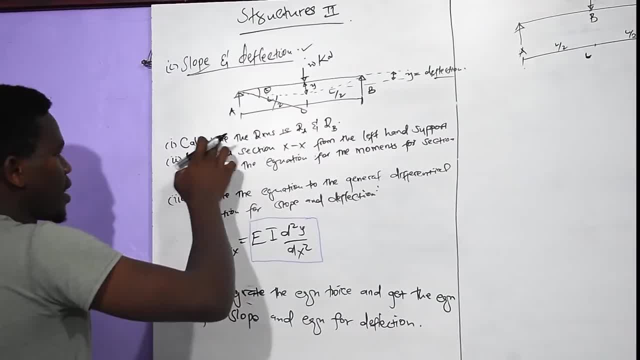 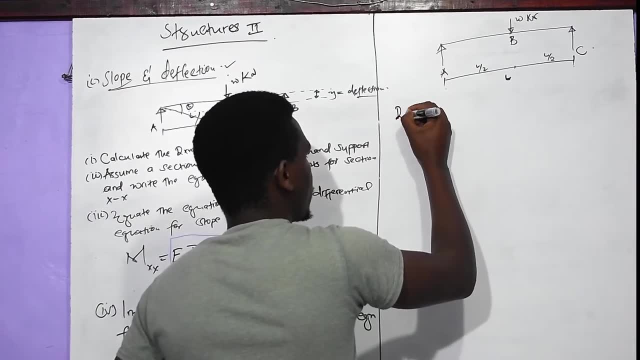 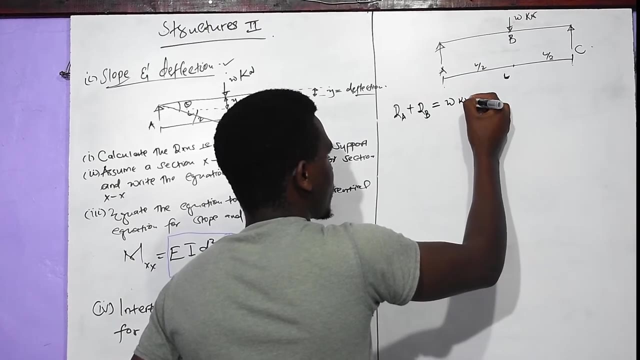 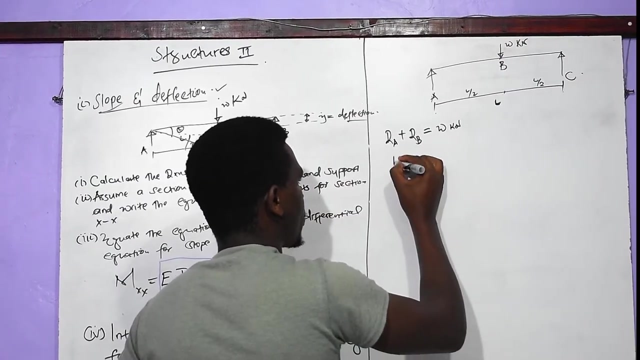 Therefore, we are told that we can create the reactions reaction A and reaction B. In this case we have reaction A and reaction C. Therefore we say that reaction A plus reaction B equals to the total loading of the beam. Therefore, since it is acting on the mid-span of the beam, reaction A will be equal to W over 2,. 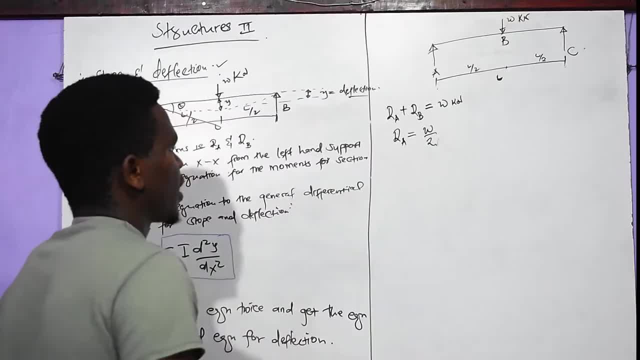 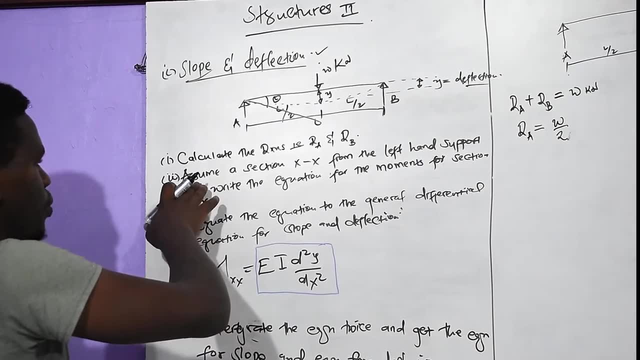 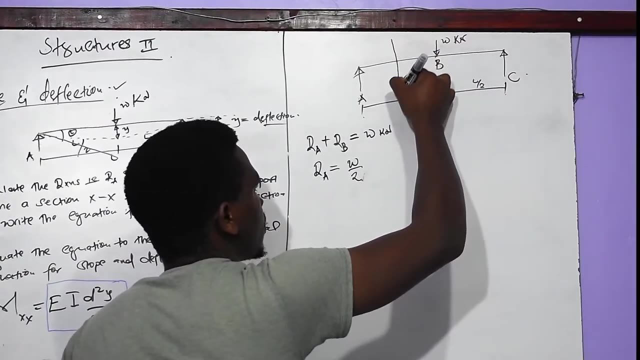 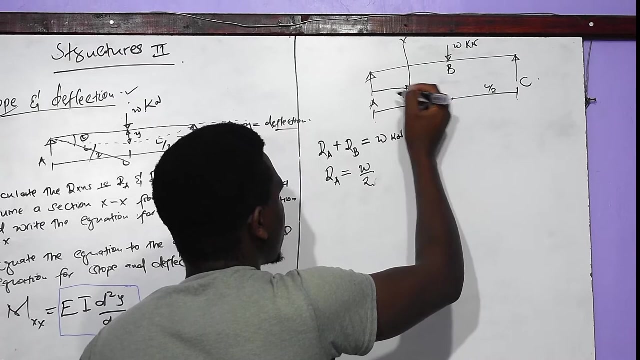 since they are equally sharing the loading. Therefore, step number 2, we are told that we assume a section XX from the left-hand support. So we assume a section XX from the left-hand support. This distance is X, like so. 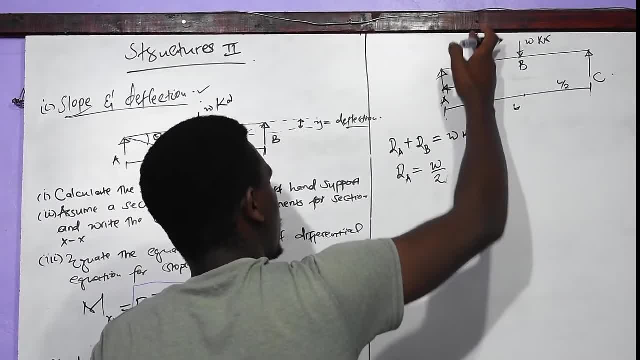 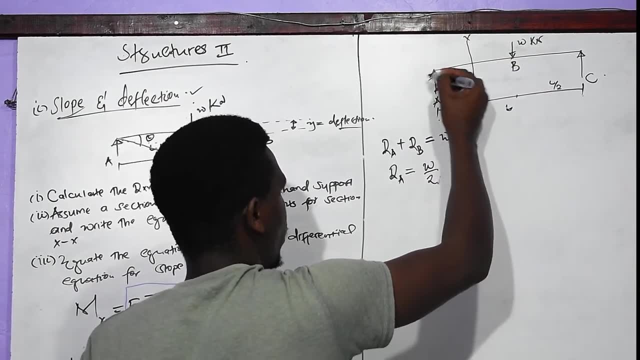 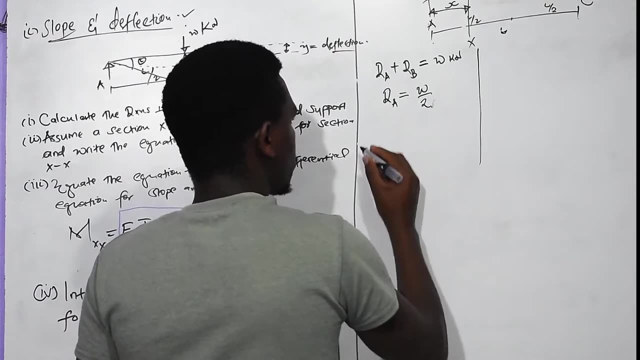 So the moment of these points, section XX, remember, moments are given by the loading times, the distance. Therefore, it will be this: This reaction A turns this distance, But we know that reaction A is W over 2.. Therefore, 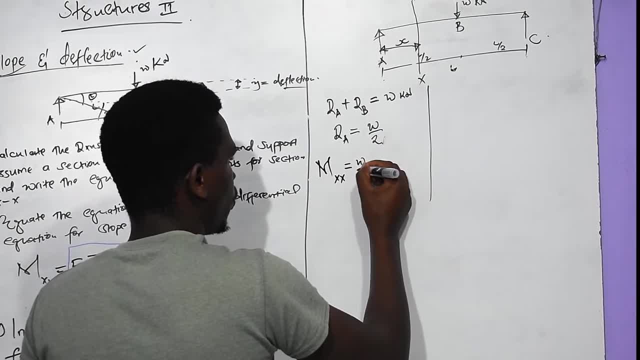 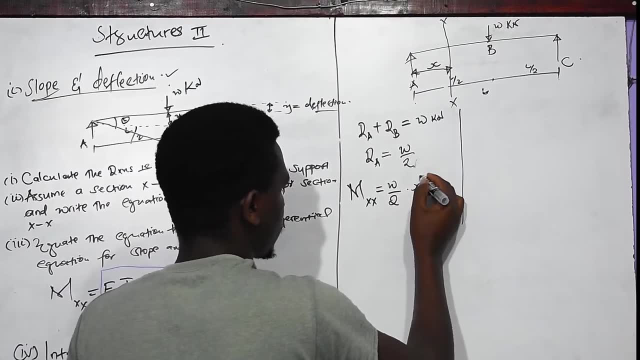 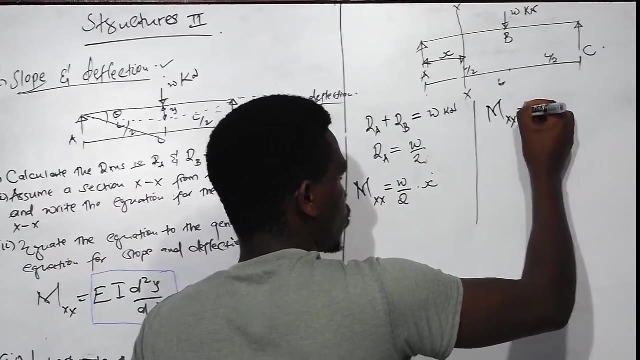 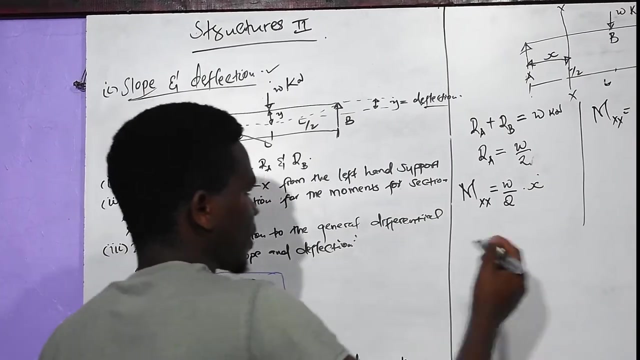 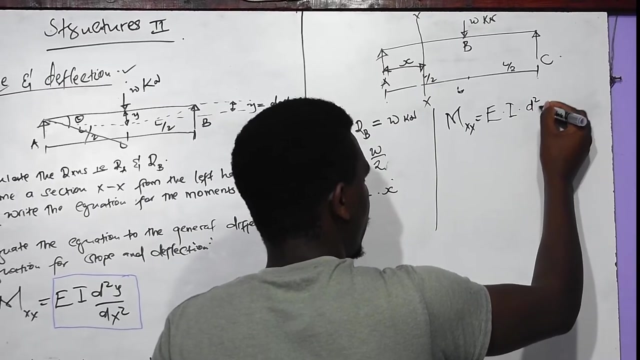 moment XX will be given by W power over 2, which is reaction A multiplied by the distance like. so. Therefore, moment XX equals to that. we should equate the equation, the general differential equation for slope and diffraction. So moment XX will be given by: E, I, B squared, Y all over DX squared. 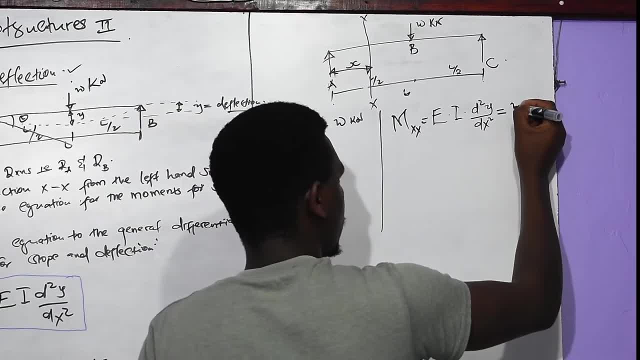 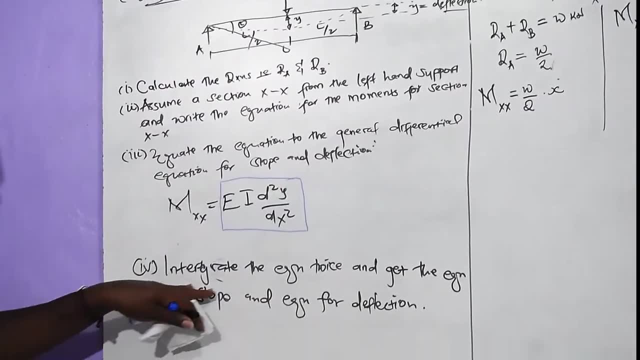 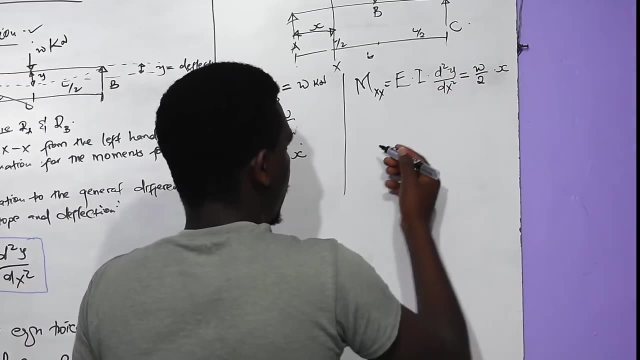 which is equal to W over 2 divided by the distance X. Step number 4, we are told to integrate the equation twice to get the equation for slope and the equation for diffraction. So if we integrate this one, integrate that one. 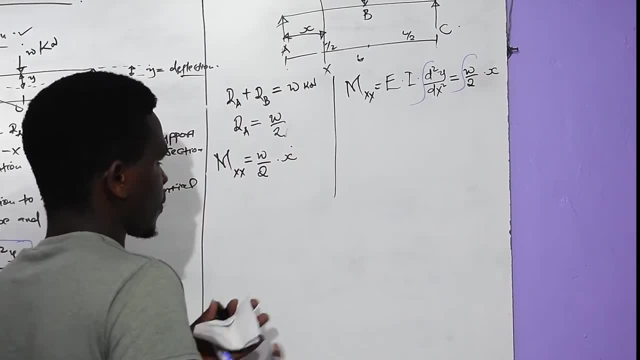 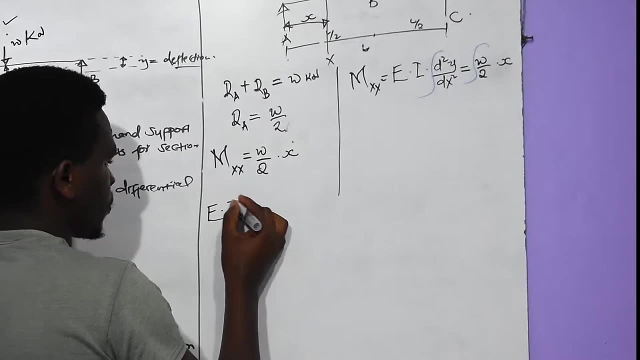 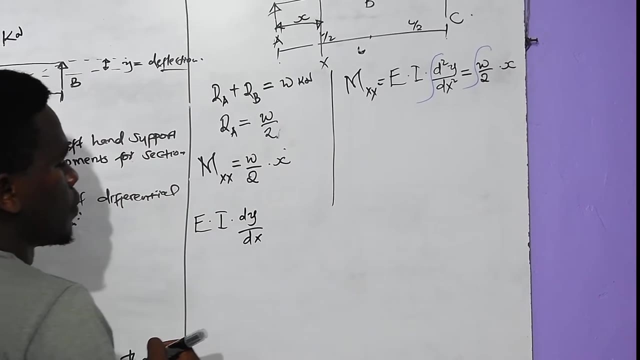 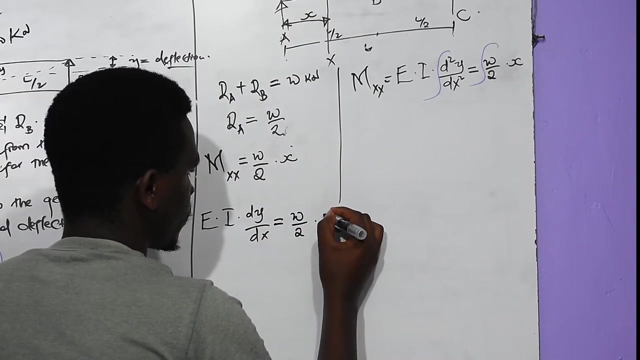 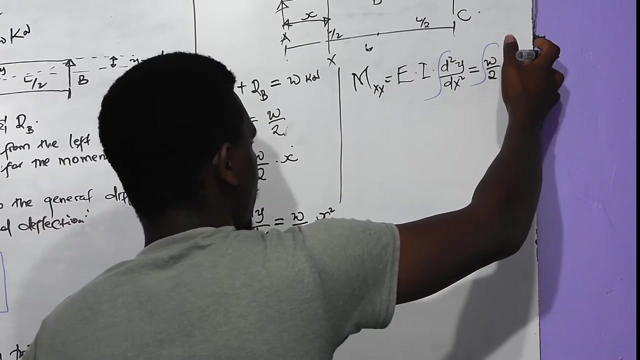 integrate that. Therefore, this one you will get. when you integrate this one, you get D I all over. DX equals to W over 2 X, squared all over 2.. Remember, when you are integrating, you add the power by 1,. 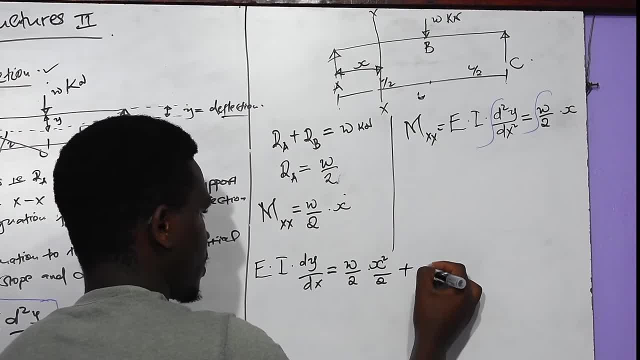 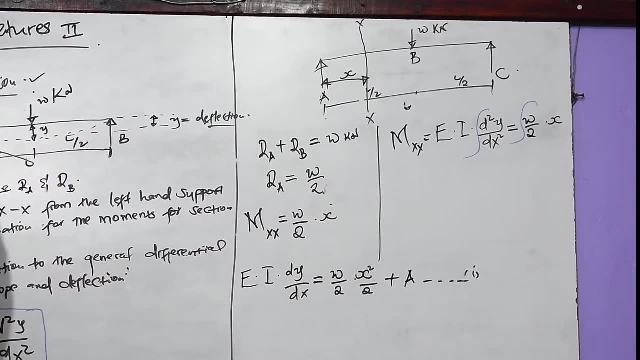 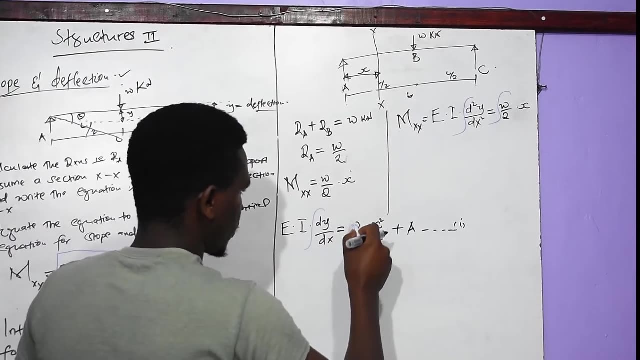 and then you divide by the new power and then you add the constant of integration, like so. That is equation 1.. So we are told to integrate twice. So we integrate this one again. So we integrate this, We integrate this, like so. 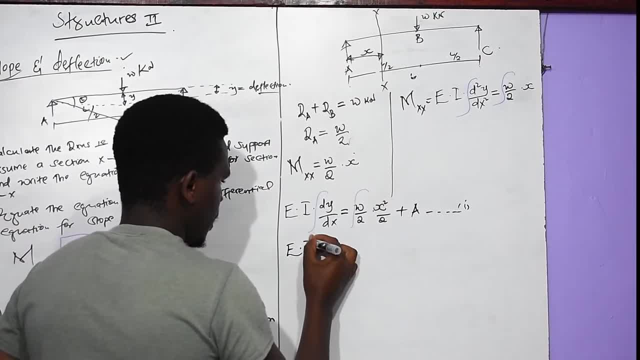 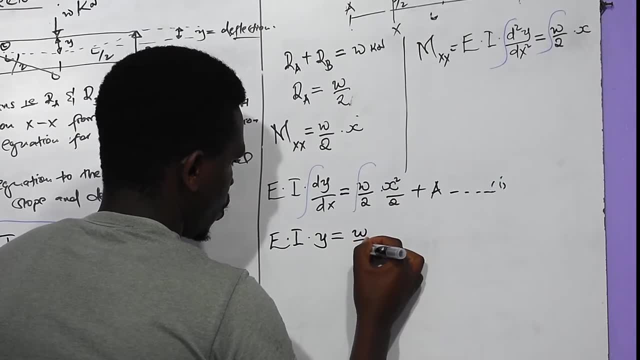 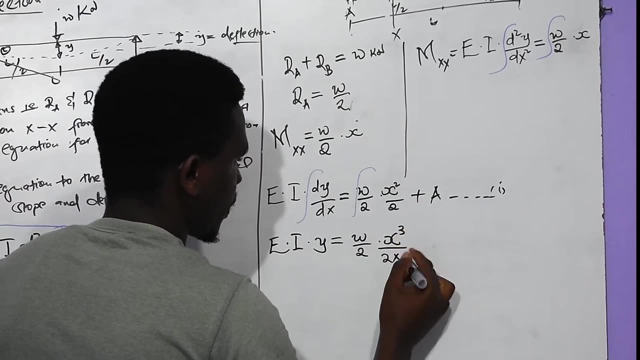 Therefore, this one will be E I. Y equals to W all over 2, X cubed all over 2, times the new power 3.. Like so, Remember we had a 2. So that is our 2.. 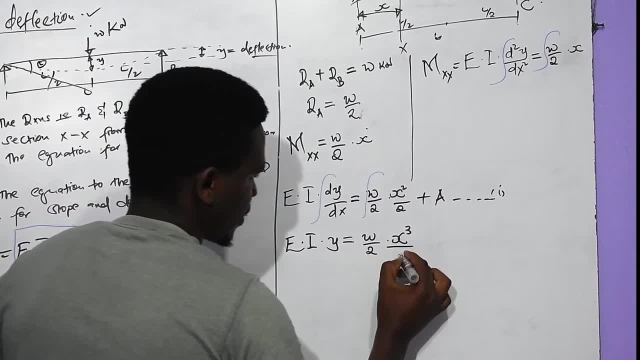 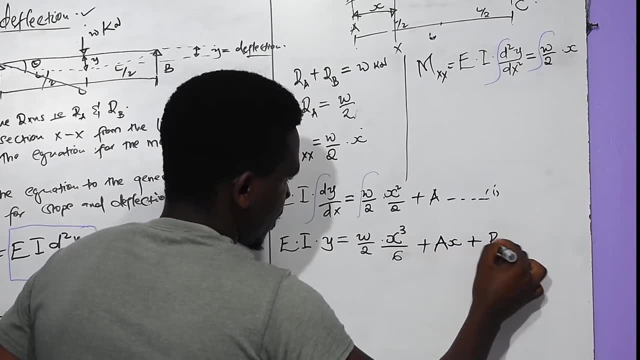 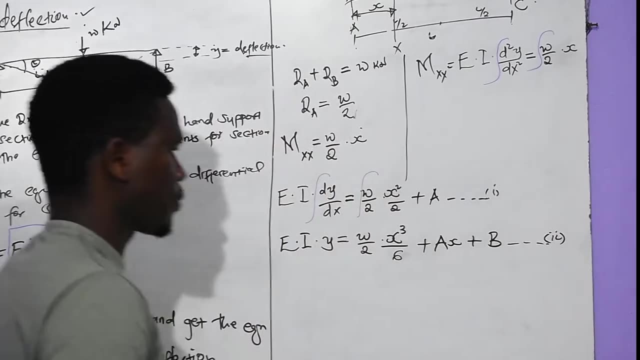 And then we divide by the new power: 3. But instead of writing that, you can write just this: plus AX, plus B. Remember our B now is our constant of integration, That is our equation 2. Therefore, to calculate, 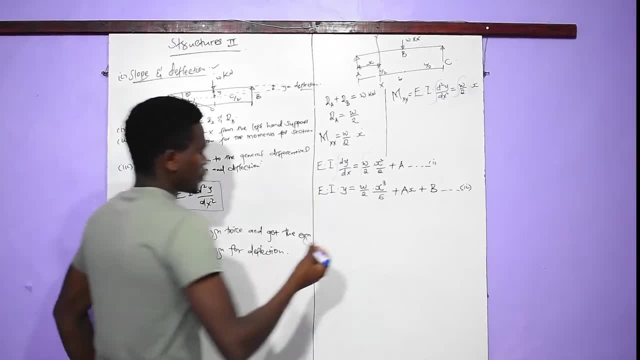 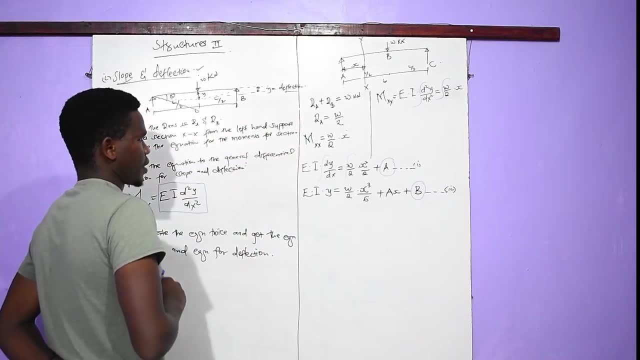 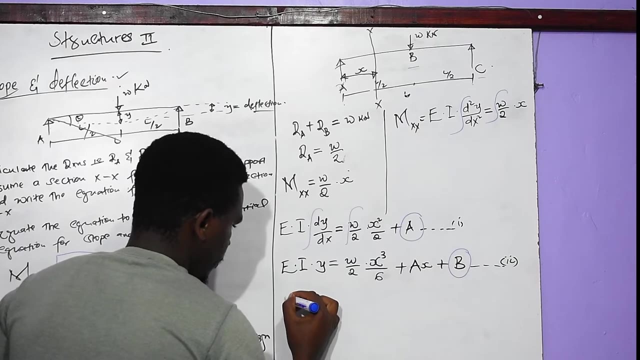 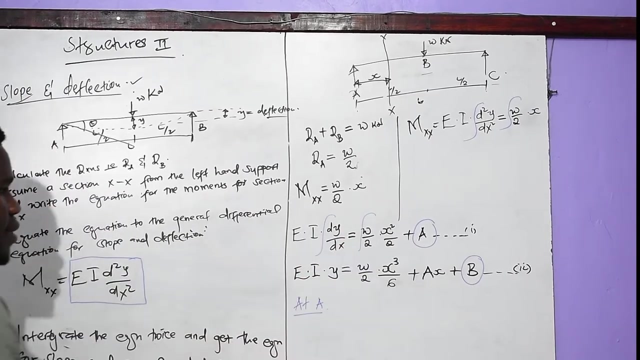 to calculate the value of A and B. A and B, there we have to follow some boundary conditions At A, at B and at C. So when at A, at A, remember our DY: DX is the slope, Y is the. 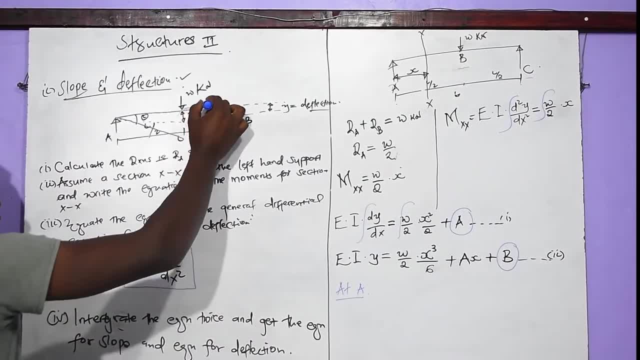 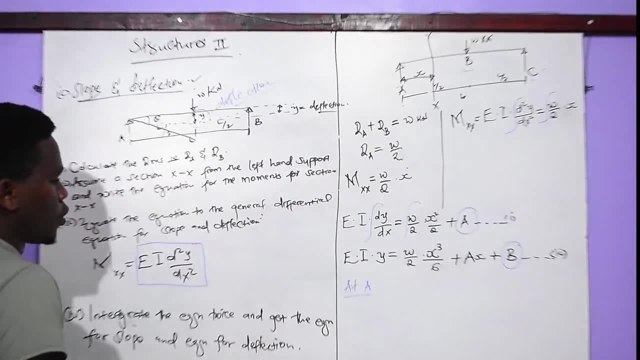 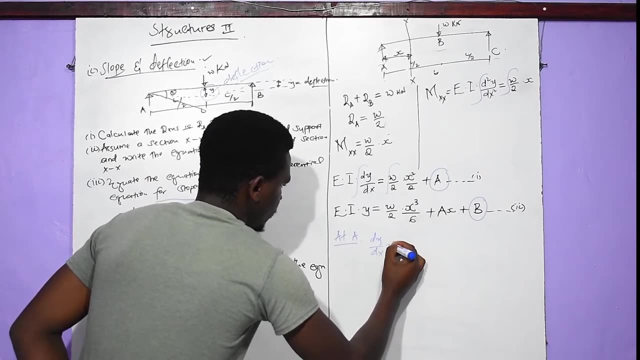 is the diffraction, as we said earlier here, But our Y here is the diffraction, Like so. So we need to know what's our DY all over DX. DY over DX at point A is theta A, Our Y is 0.. 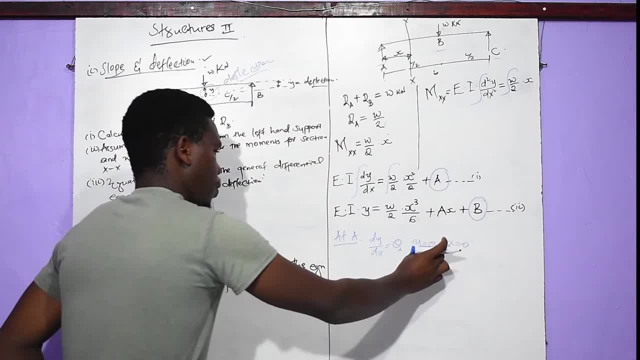 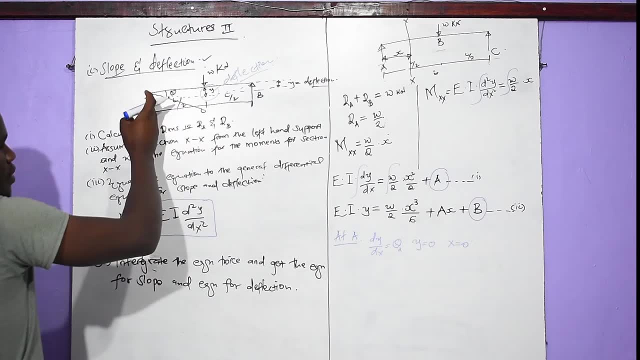 Y. Our Y here is the diffraction. At point A we do not have any diffraction. You only have the slope, And therefore our Y is 0.. For our X to be 0,, therefore you are considering from that. 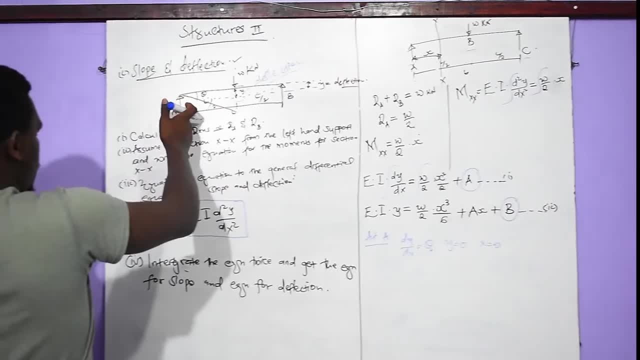 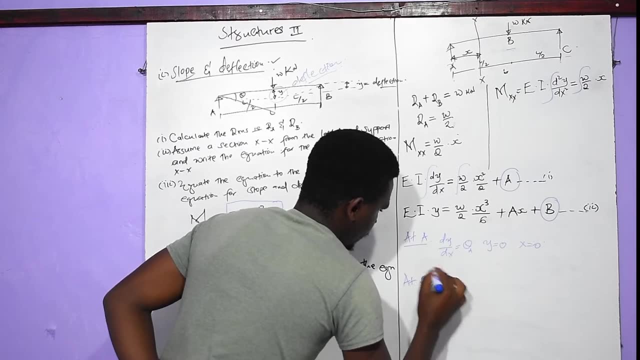 that place where you are. you are calculating from towards the left. We do not have any distance to the left. Therefore our X is 0.. We go at B When we come here at B. remember B is here, It is at the centre of the beam. 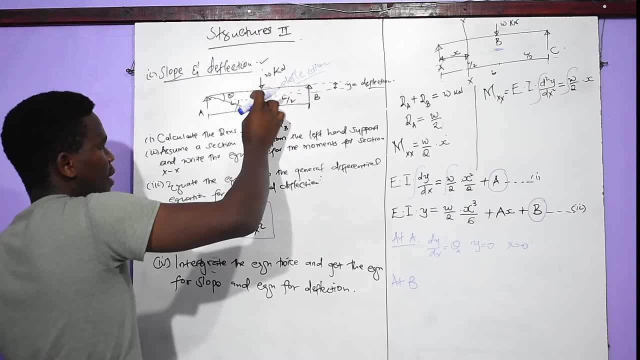 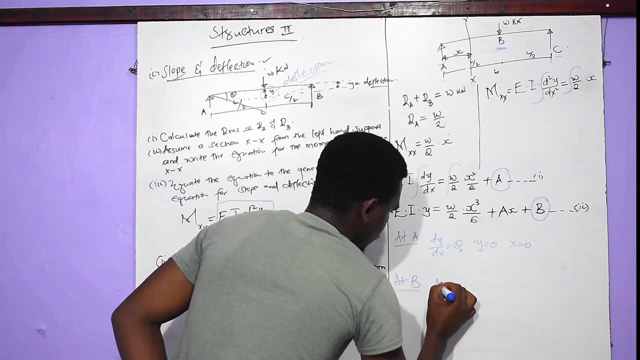 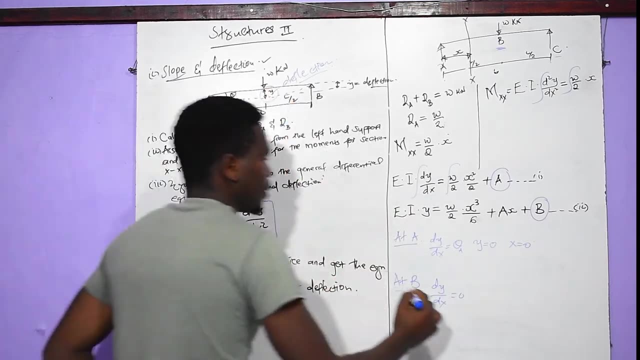 At B we have, the Y is maximum because that is where the beam is loaded. So our DY all over DX, which is our slope, equals to 0.. We do not have any slope at the centre. Our Y equals to maximum. 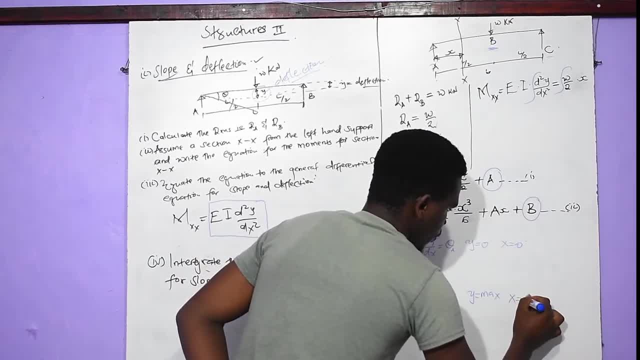 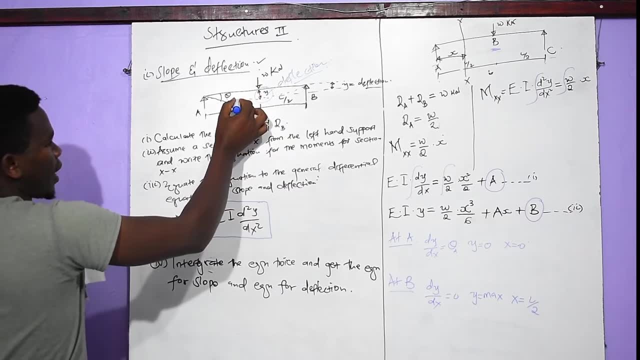 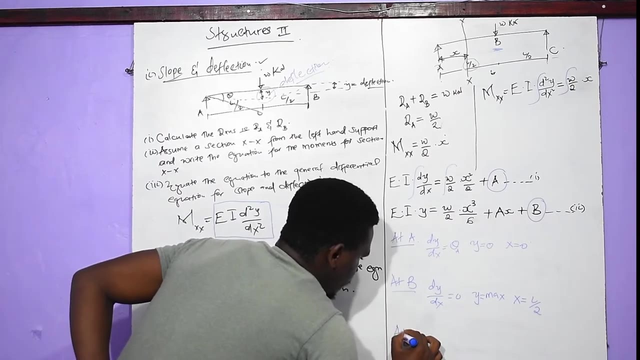 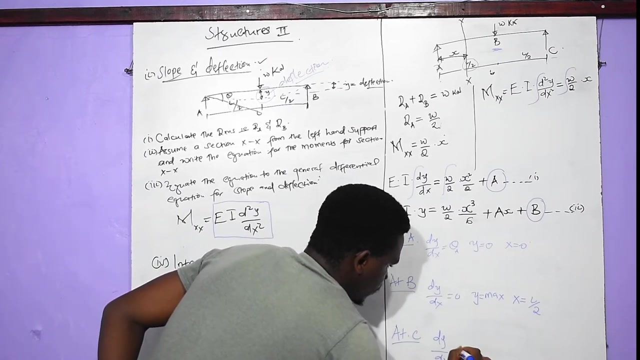 And our X equals to L over 2.. Why We are considering from that point towards the left. So from here towards the left, our L is L over 2.. This one here Like. so We go at C DY all over. DX equals theta C. 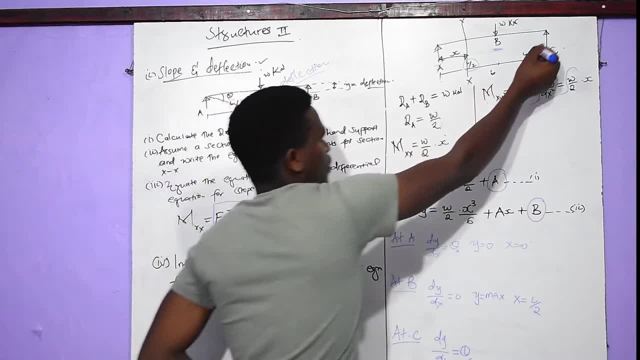 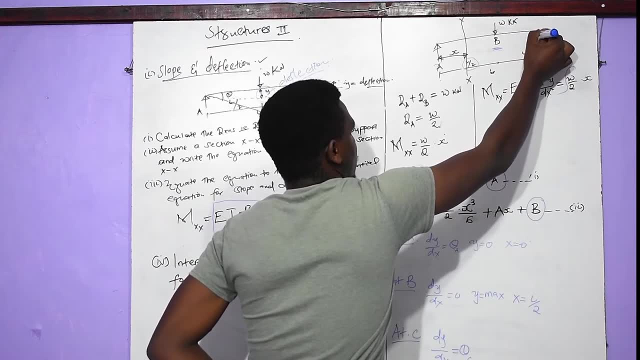 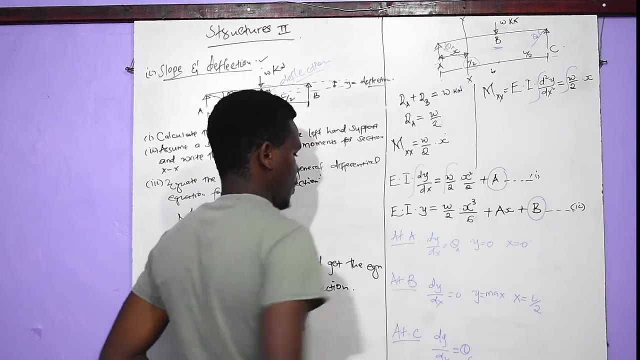 Like so We have the slope at this point here, At this point here, Like so, Since this one tends to have this theta here, our theta is C And this is our theta: A. Like so Y equals to 0.. 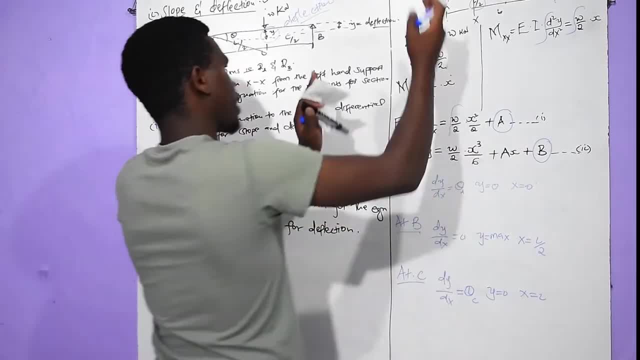 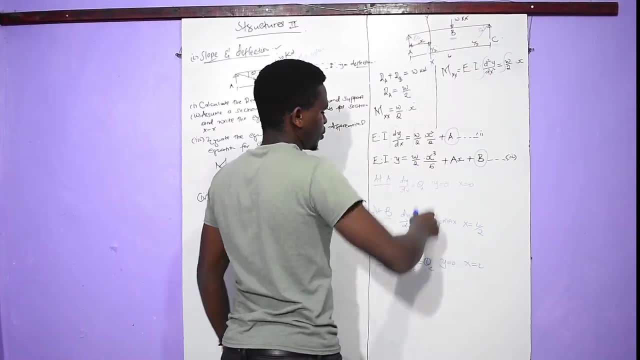 And our X equals to L. Remember, we are considering from that point towards the left. Therefore, from here to here is our L. Remember this one is L over 2.. This is L over 2. Like, so, Therefore, for us to calculate the value of A. 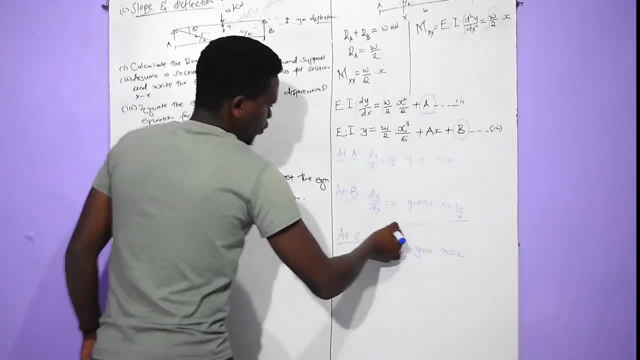 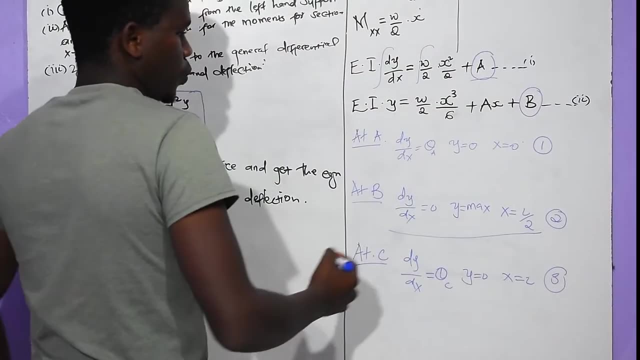 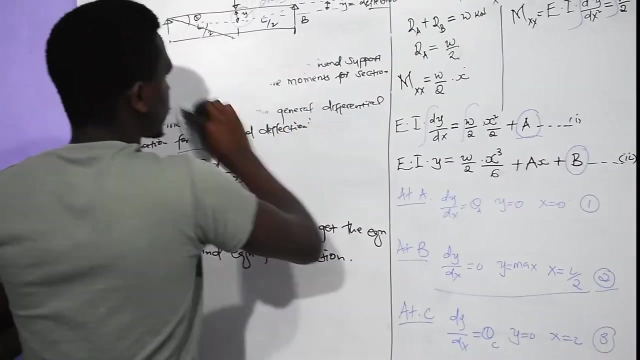 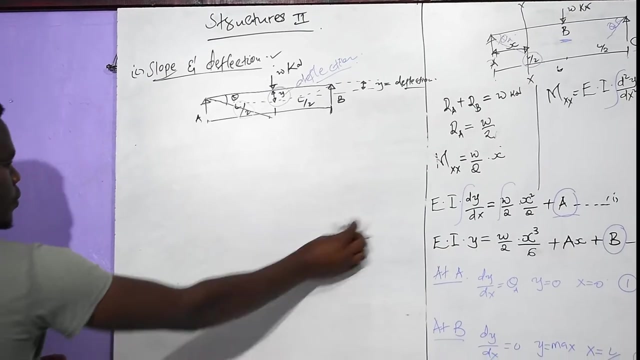 apply boundary condition 2.. We can see that this is boundary condition 2, boundary condition 1, and boundary condition 3.. So we apply boundary condition 2 in equation 1.. Yeah, So apply boundary condition 2 in equation 1.. 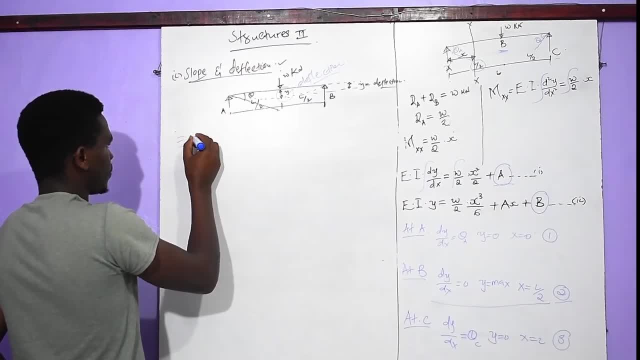 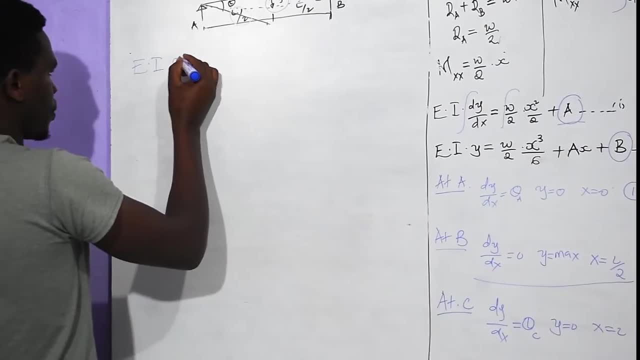 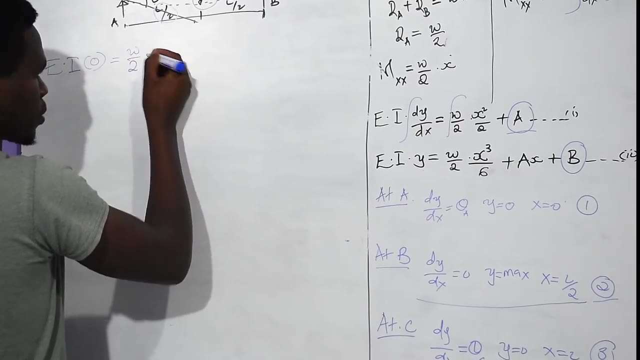 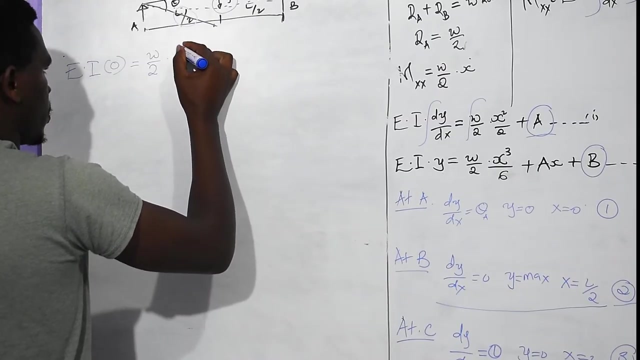 We get EI over DY over DX. DY over DX is 0.. So we put a 0.. Equals to W over 2.. X squared. Our X is L over 2.. So L over 2.. This one is squared. 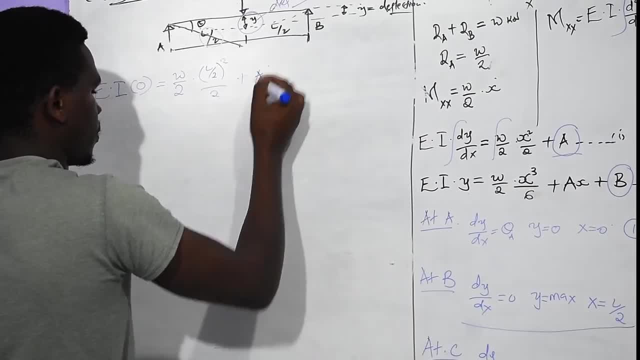 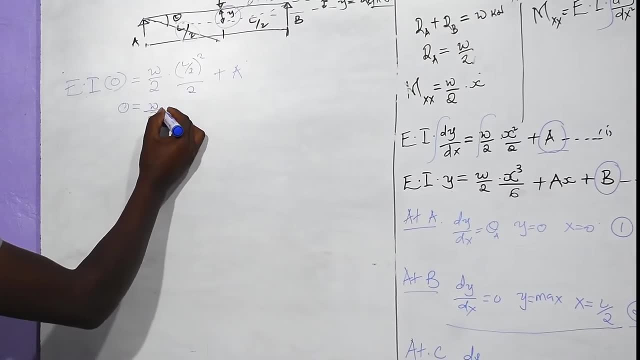 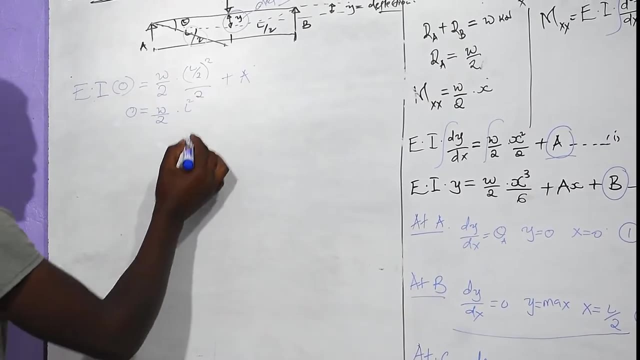 1 over 2.. Plus A Like so. So this one we get is 0.. Equals to W over 2.. This is L squared, 2 squared, that's 4.. 4 multiplied by 2,, that's 8.. 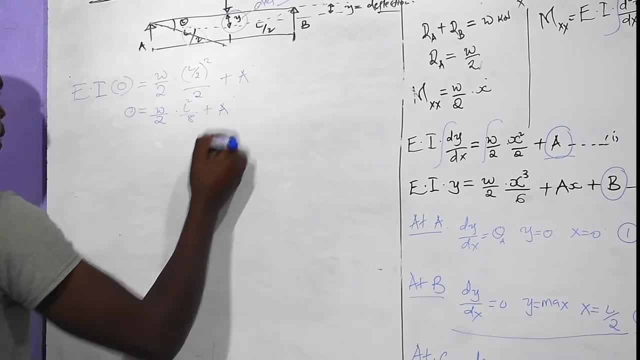 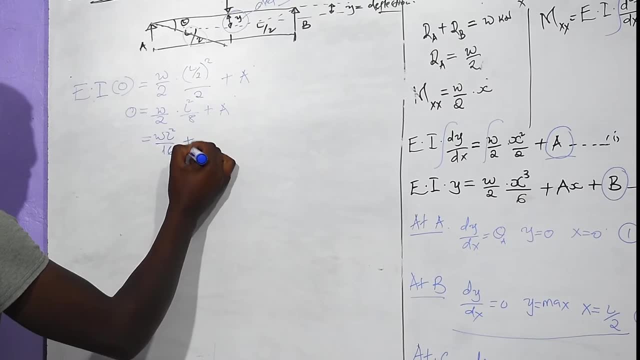 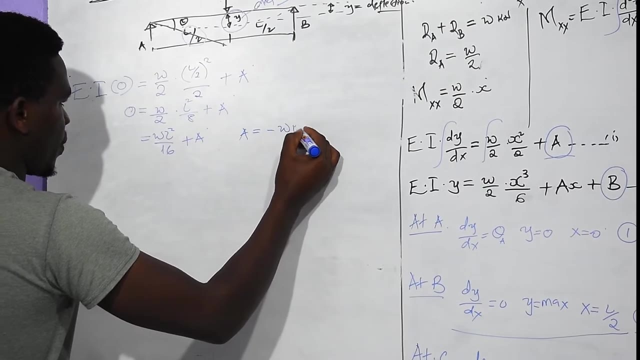 Like so Plus A: Yeah, So this one we get is WL squared 1 over 16.. Plus A: Take this one to the other side. Therefore, we get that A equals negative WL squared All over 16.. 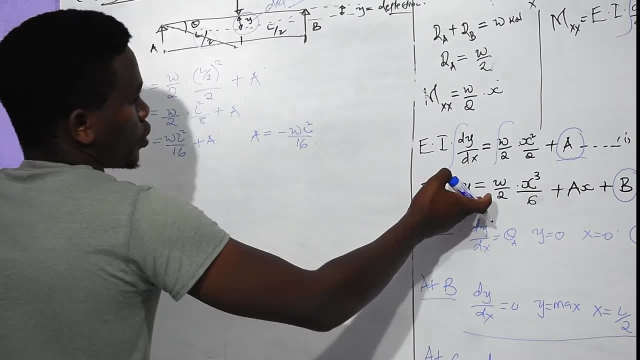 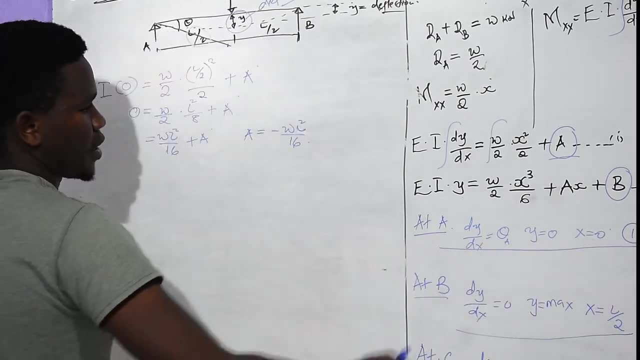 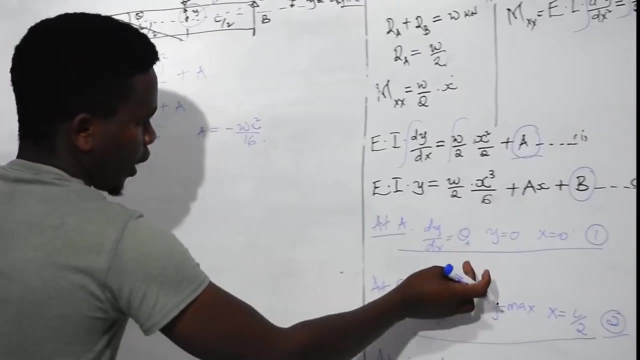 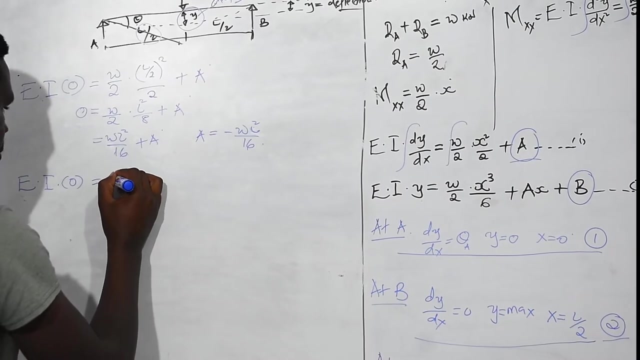 Like. so We go to equation 2.. We take boundary condition 1.. We apply it in equation 2.. Therefore, this one will be EI. Our Y is 0.. So we put a 0 there Equals to W over 2.. 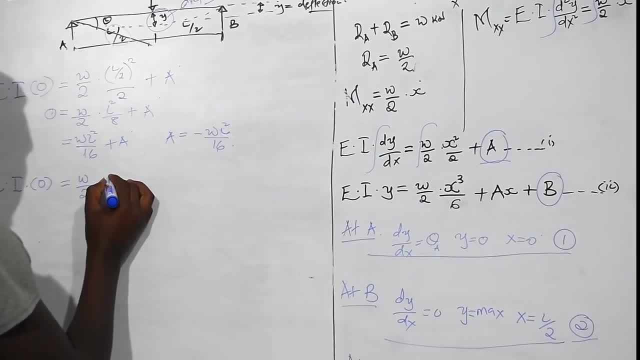 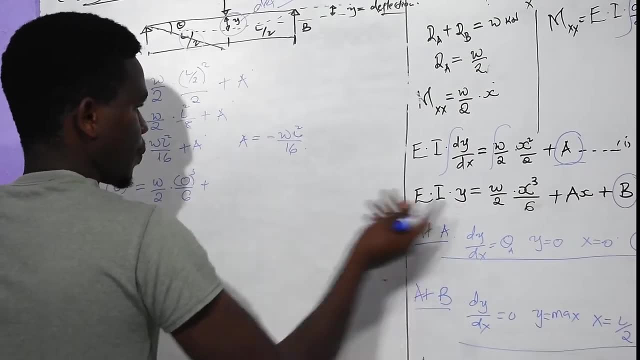 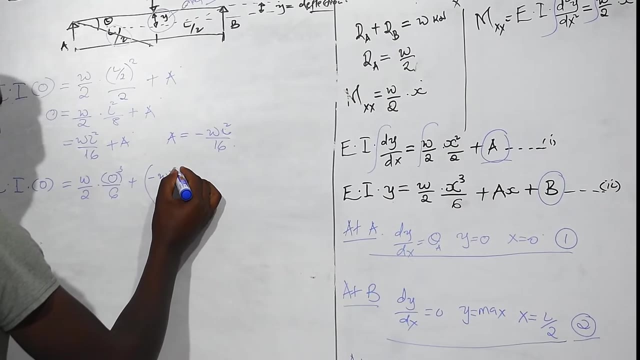 Our X here is X is 0.. So we put a 0.. So that means WL squared Y over 16.. All over 16.. Plus We have AX. We know that our A is this one, So plus into brackets. 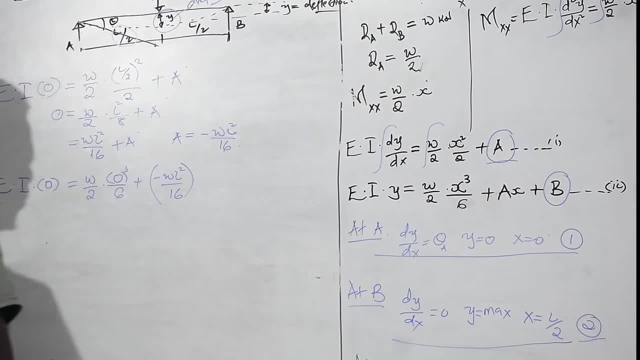 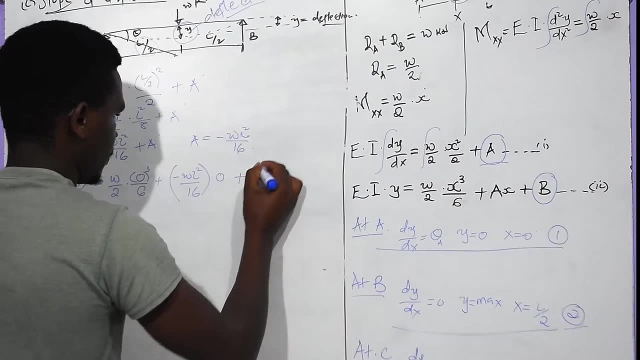 Minus WL, squared All over 16.. Like so You multiply by X, But our X is 0. So we put a 0 there Plus B Like, so This one will be 0.. This one will be 0.. 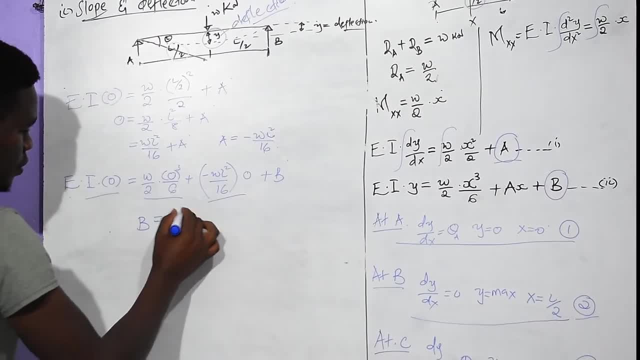 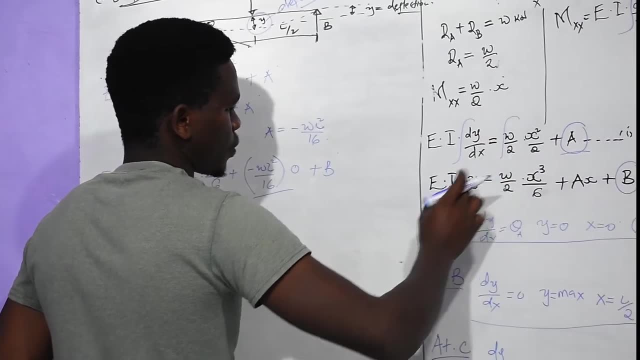 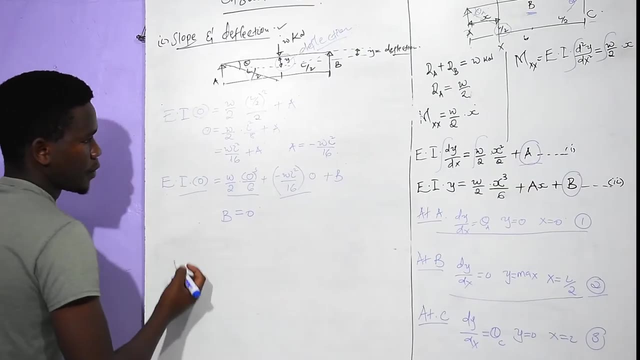 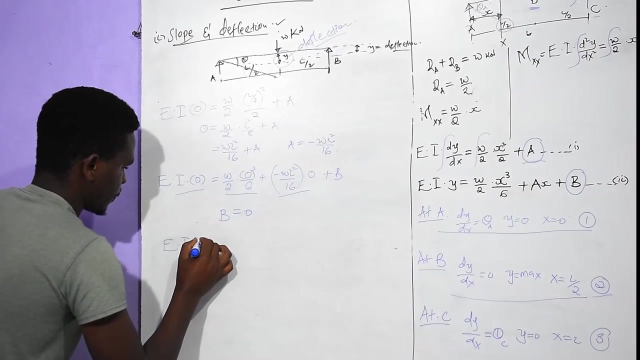 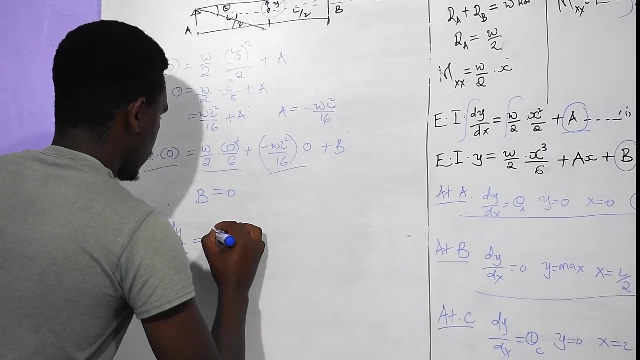 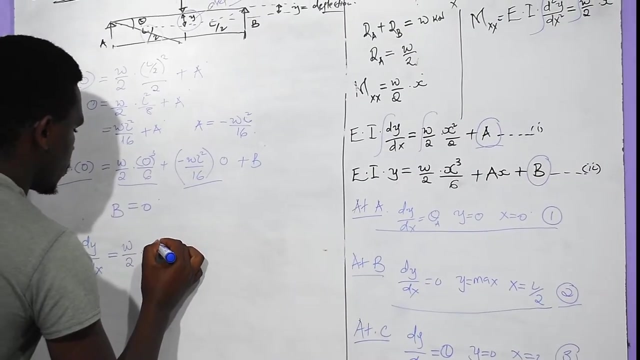 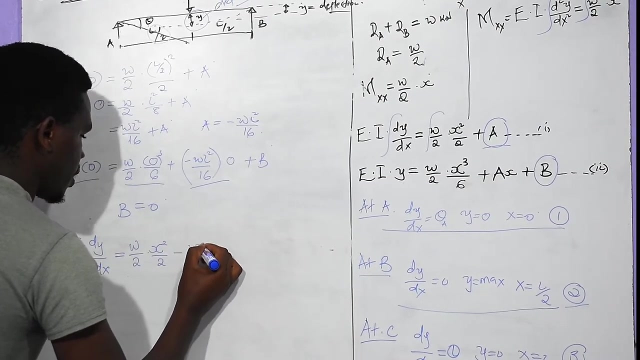 This one will be 0.. and therefore b equals to zero, like so. so from there you write, you rewrite the equations, equation one and two, inserting the correct values of the exact values of a and b. therefore, it will give us a to avoid the value of a, so it will be negative. w l squared. 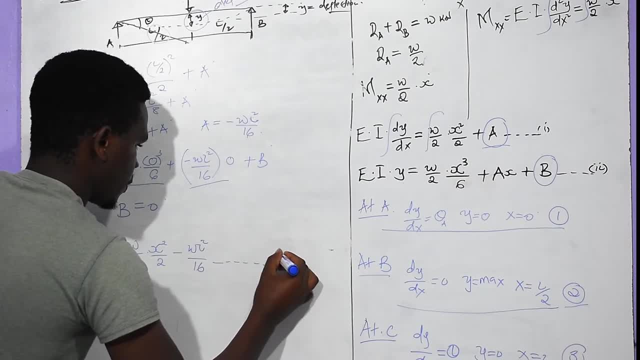 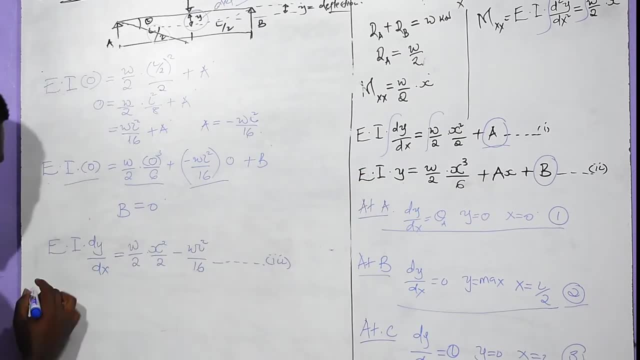 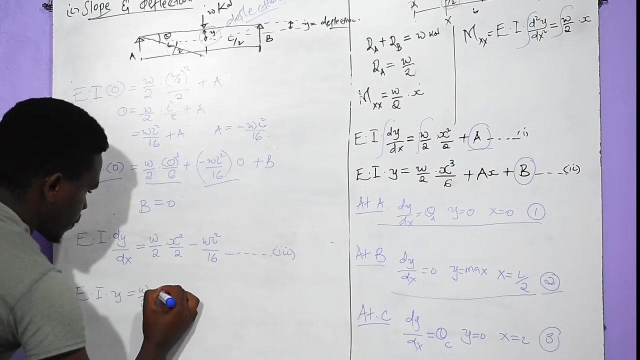 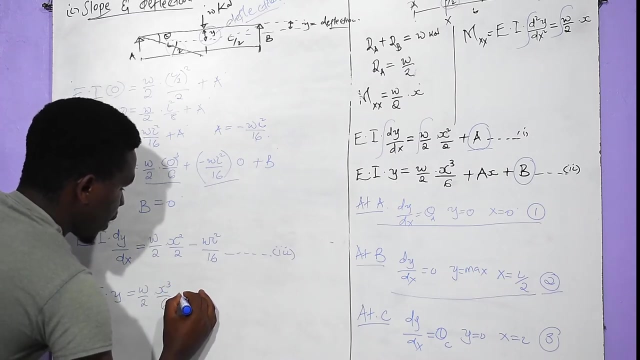 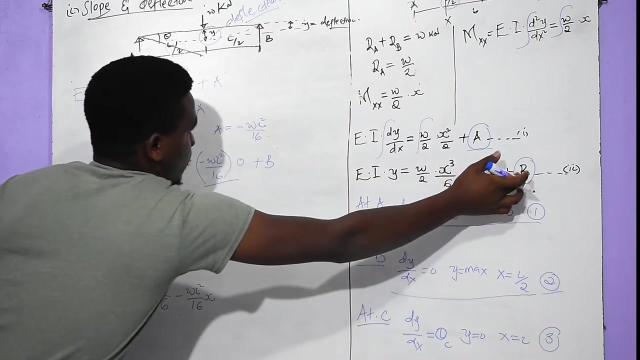 all over 16, and this is our equation three like so, uh, for the equation two she'll give us: i y equals to w over two, x cubed over six minus. remember this: a is this one: w l squared over 16, multiplied by x squared over six. 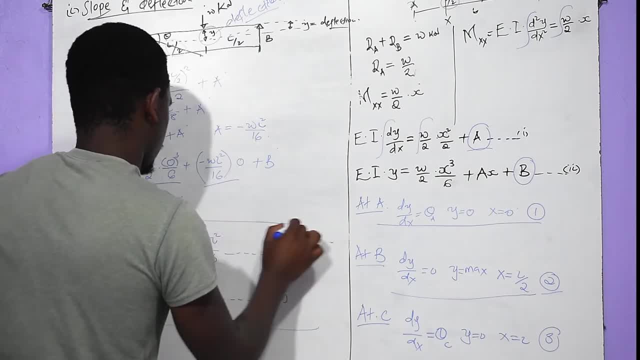 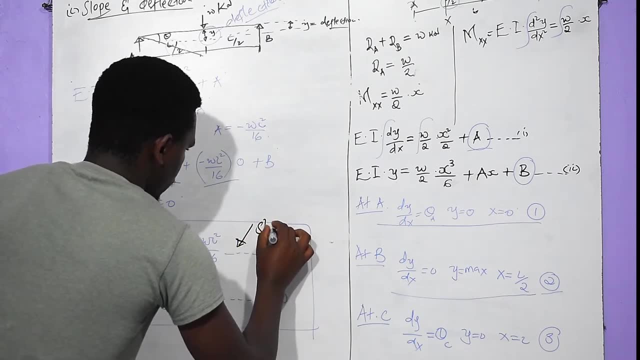 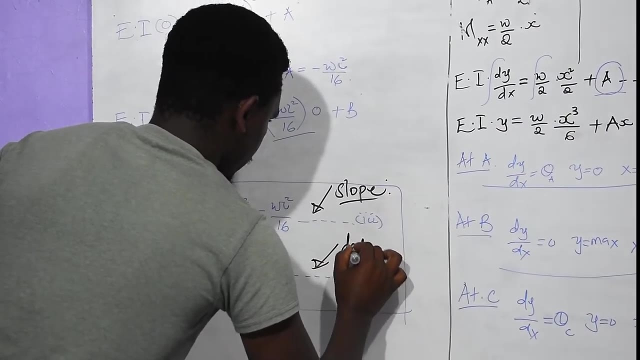 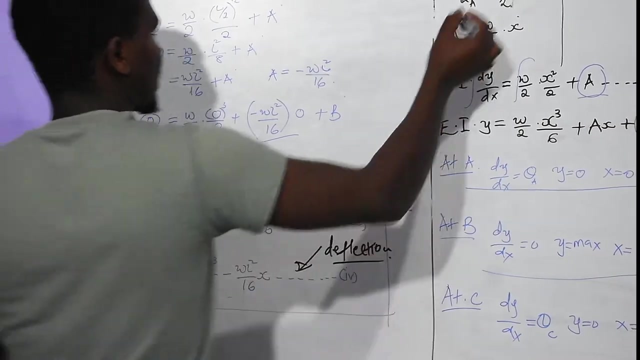 remember, b is zero, so it is okay that way and that's one equation. four and up to there we have the two equations and therefore this is the equation for slope and this is the equation. So we need to calculate the slope at A, slope at C and diffraction at B. 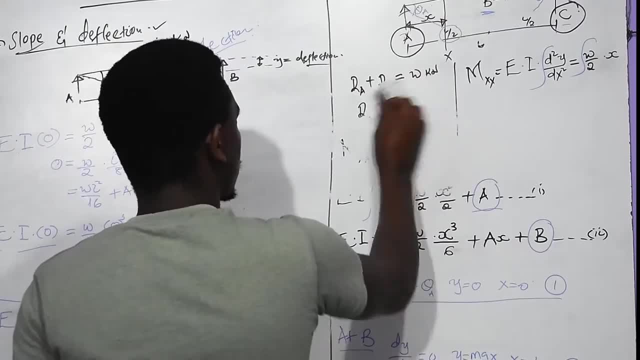 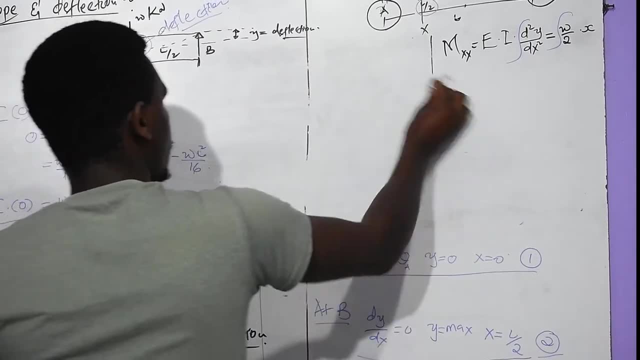 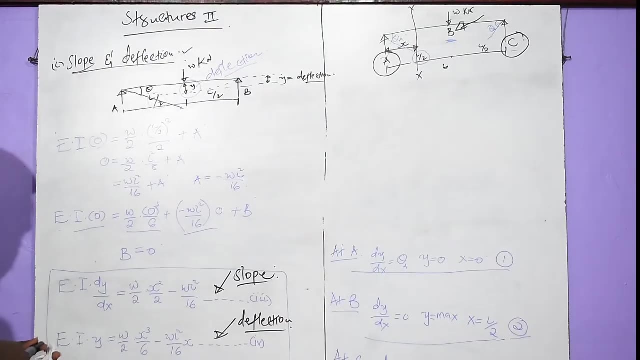 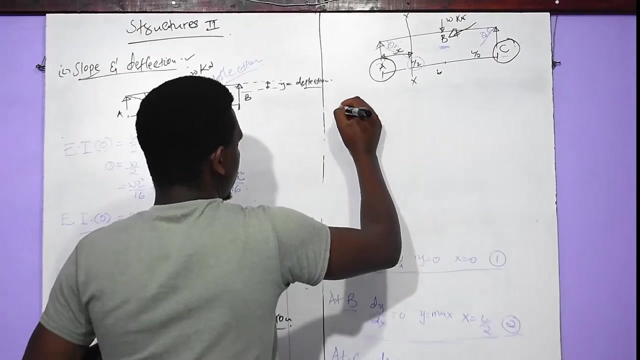 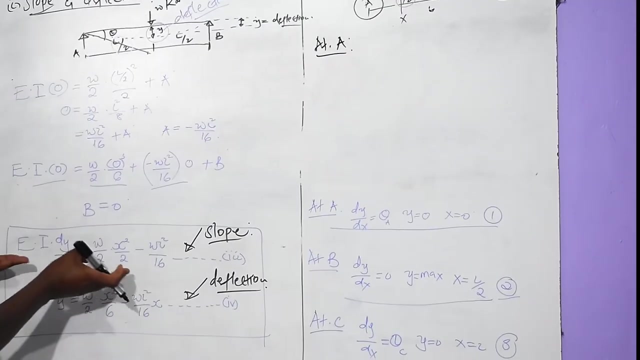 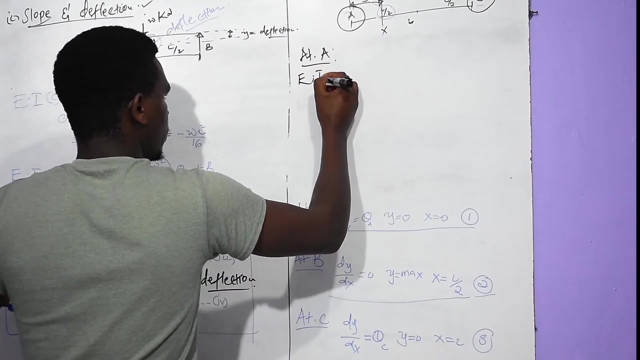 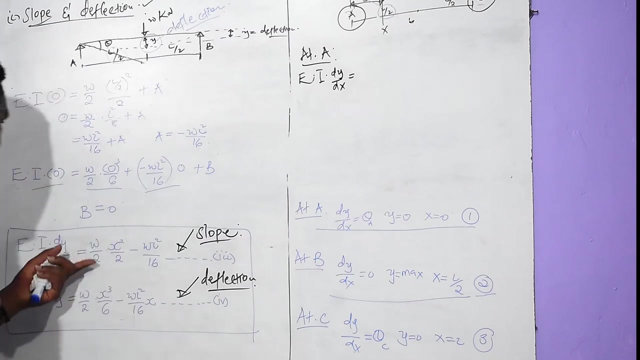 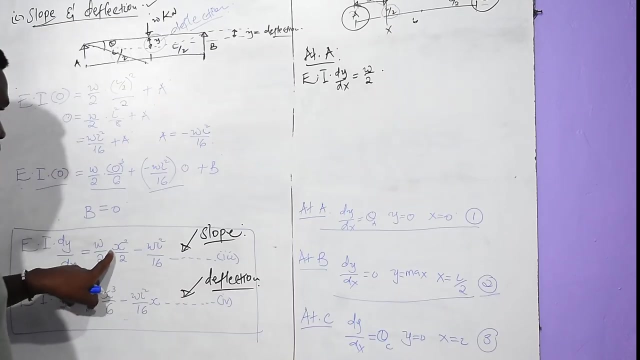 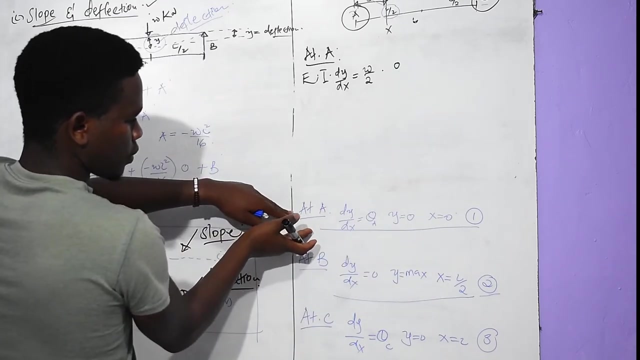 Like so. So let's see, Do not want to erase the boundary conditions, Do not want to erase the boundary conditions, So we will be given by W over 2 dot. our X in this case is 0.. So use boundary condition 1 at A, boundary condition 2 at B and boundary condition 3 at C. 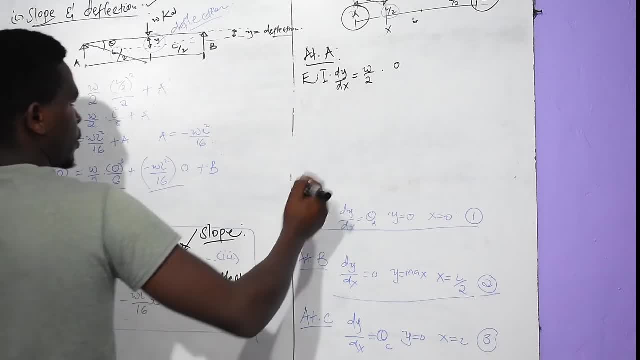 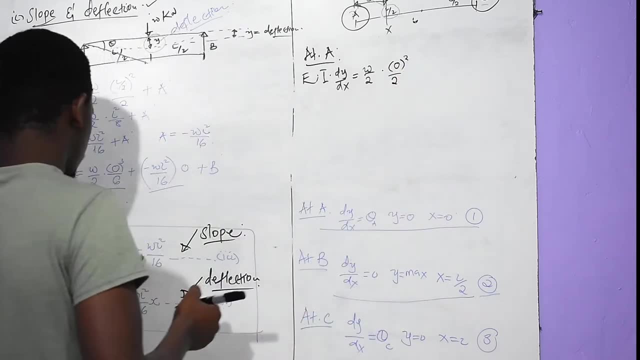 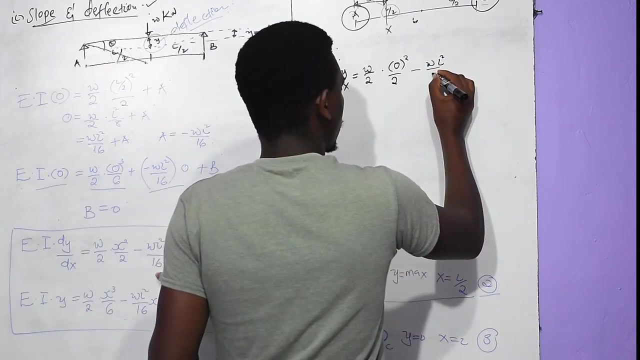 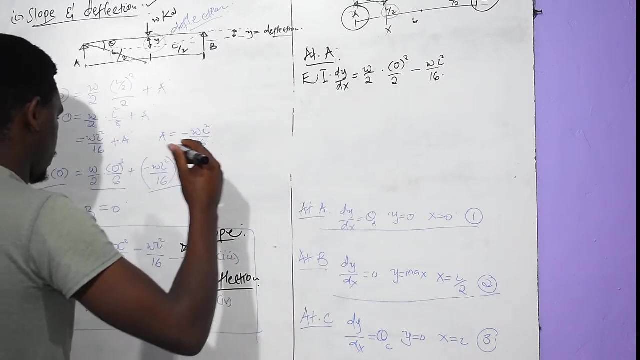 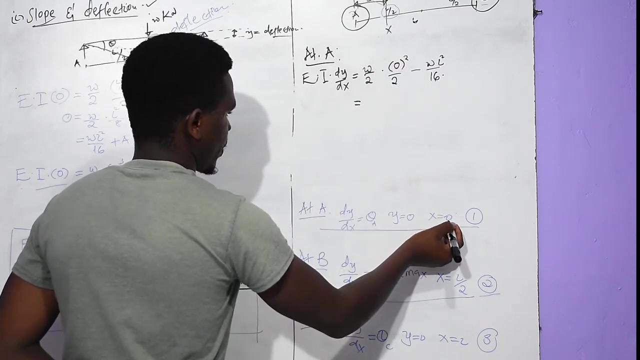 So in this case, we are going to use boundary condition 1 at A Like. so Minus 3L squared over 60. Like. so, Therefore, this one will give us this one will be 0.. Since our X, our X here was 0.. 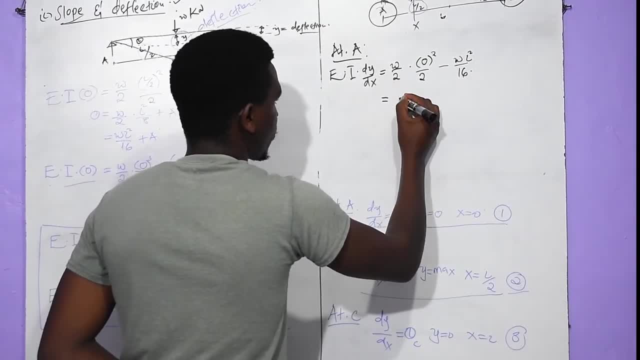 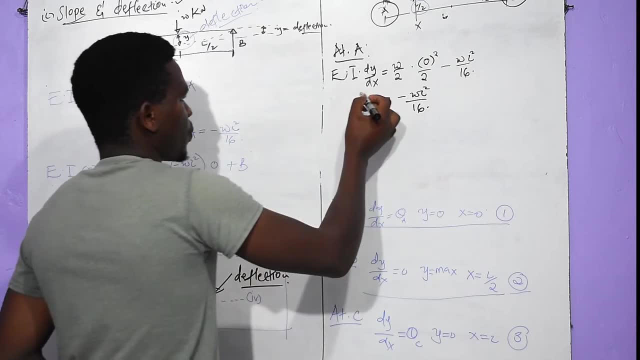 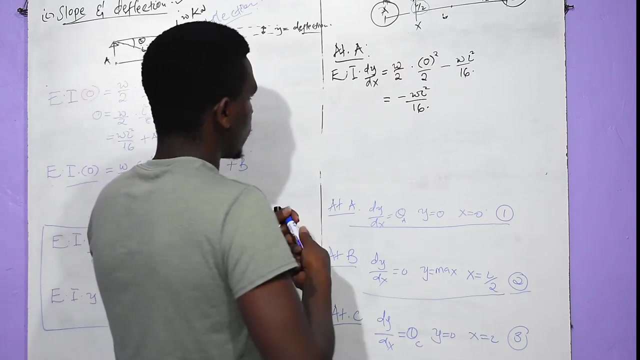 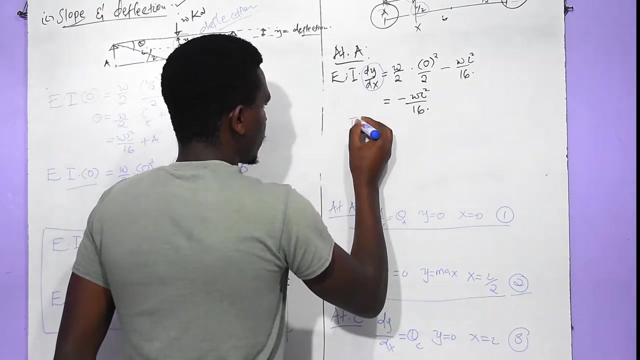 So we put a 0 here and this one will give us 0.. Therefore, this will be minus WL squared over 60.. Like so, But then we are interested. We are interested with the DY over DX, Therefore EI DY. 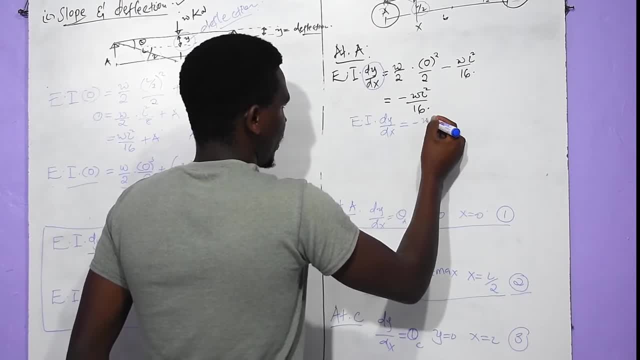 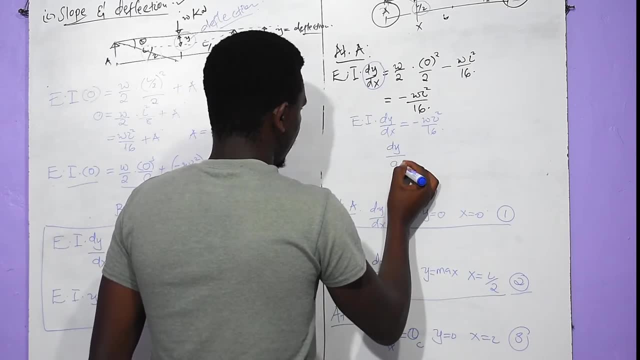 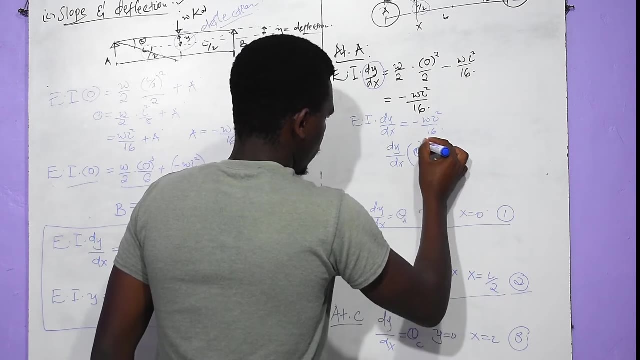 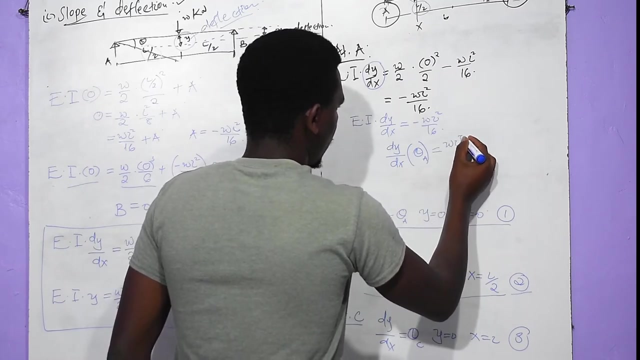 Therefore, for DX we will be given by negative WL squared over 60.. Therefore, DY for DX, which is theta, Also theta A- Remember DY over DX- denotes the slope. Therefore theta A will be given by WL squared. 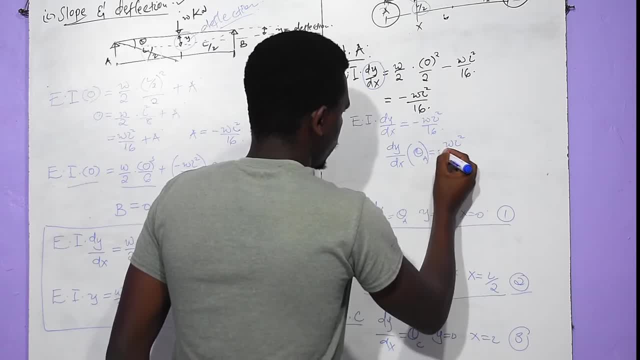 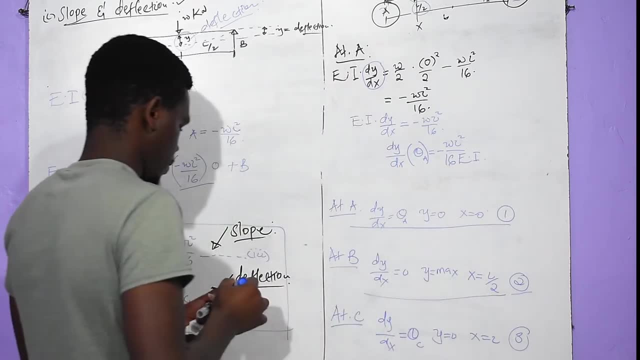 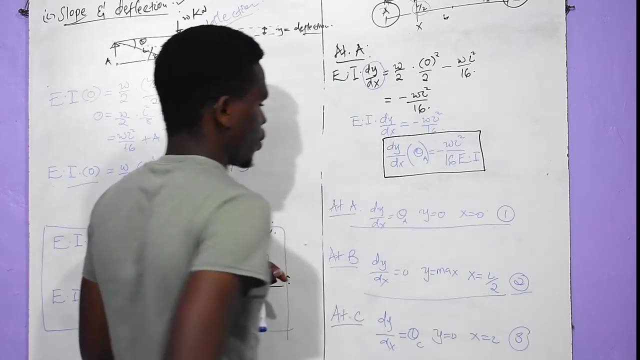 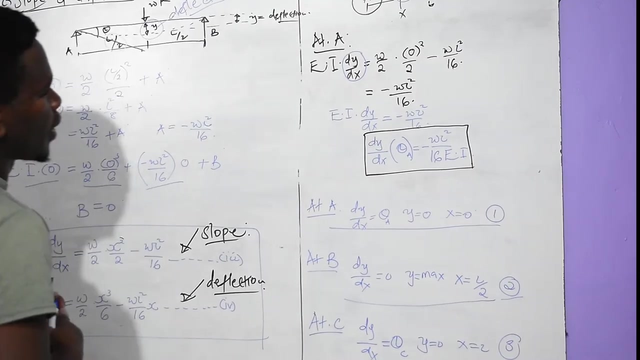 This should be negative. sorry, Cost to negative WL squared. WL squared all over 60.. EI Like so. So this is the equation for slope at A. Let's calculate slope at C. Therefore, we use the same same equation. 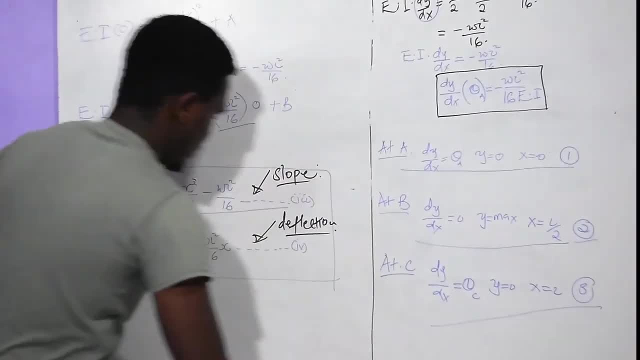 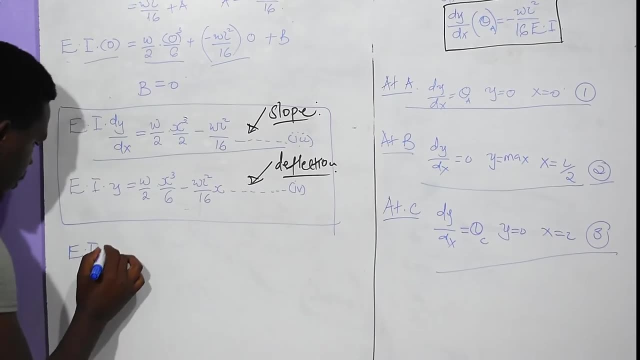 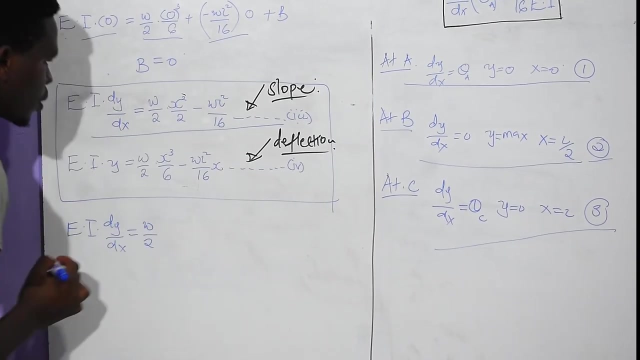 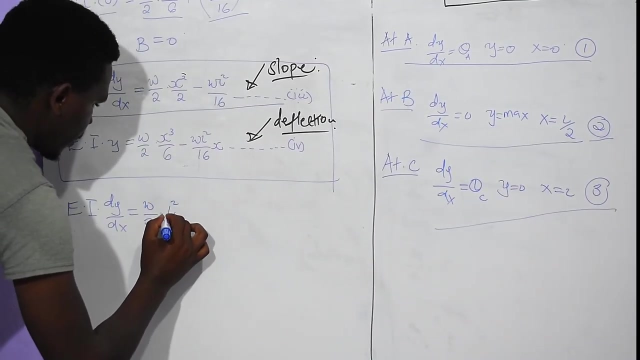 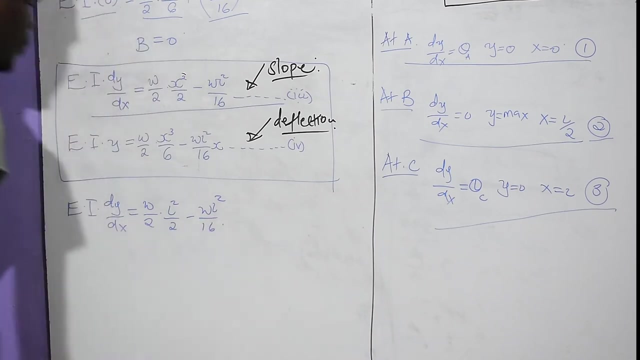 But then we use for this one 0.. What's the damn line now? 0.. at C, So this one will be EI. dy over dx equals w over 2.. Our x in this case equals L, So we put L. this one is squared 1 over 2, minus wL, squared 1 over 16.. Like so, So this one. 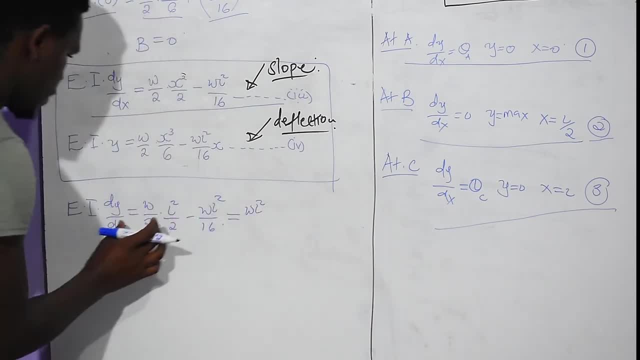 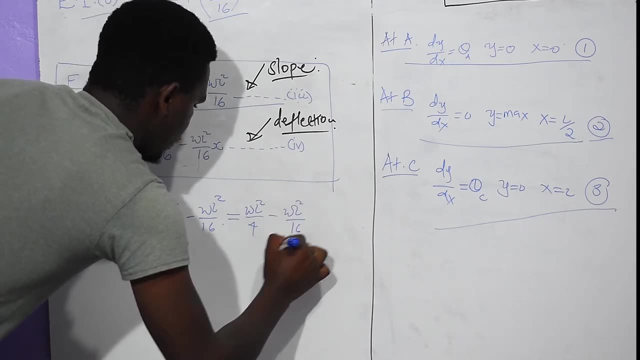 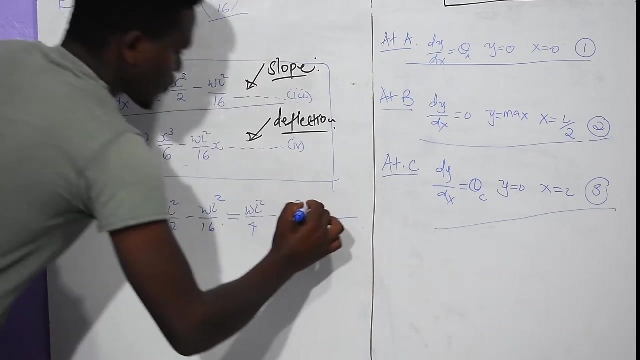 will be wL squared this one, wL squared 1 over 4, minus wL squared 1 over 16.. Like so, If you get the LCM, it will be 16.. 16 divided by 4, that's 4.. So you get 4.. So you. 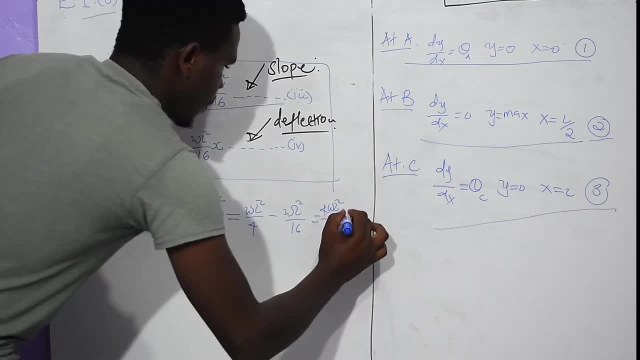 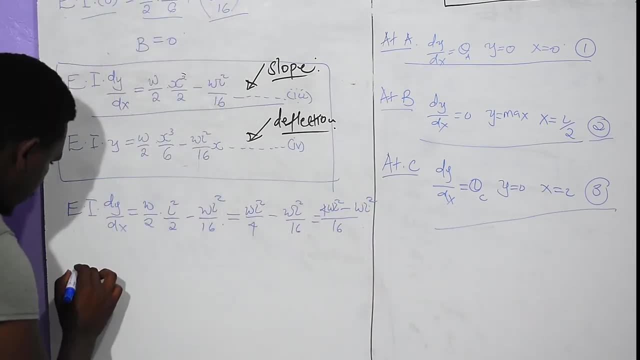 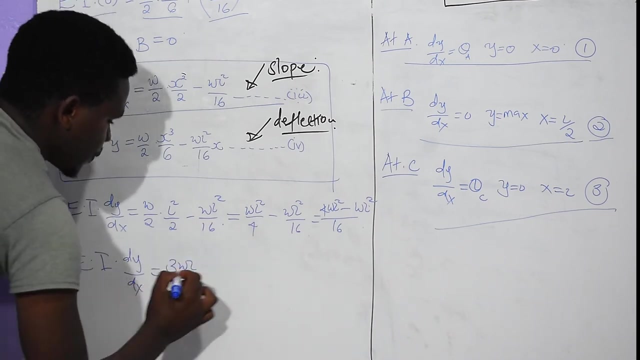 get wL squared minus this one will be 1, so wL squared Like so. Therefore, EI dy over dx will be given by this one will be 3.. Therefore, 3 wL squared over 16.. Like so. 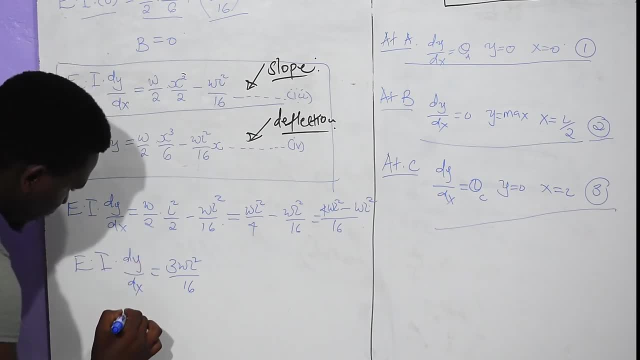 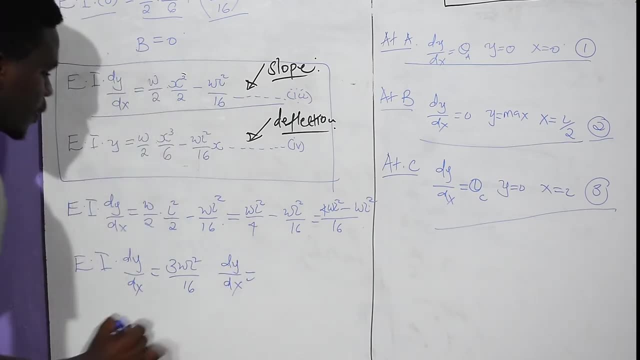 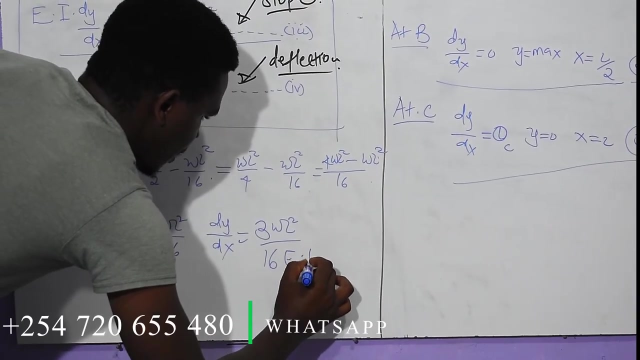 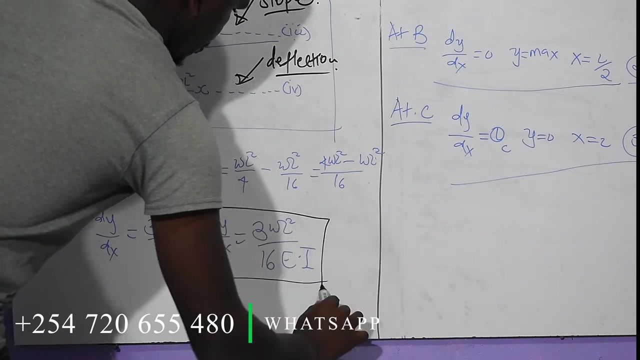 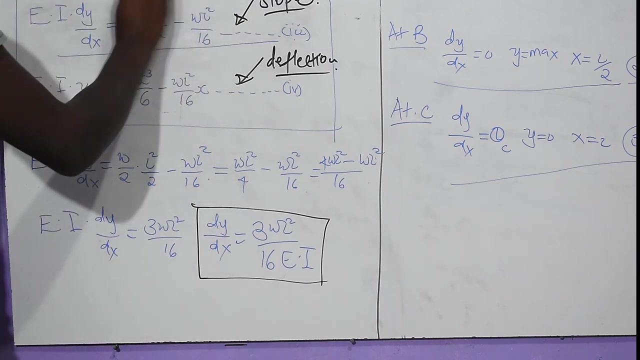 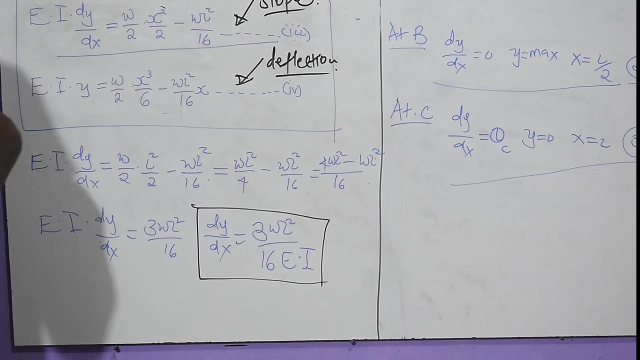 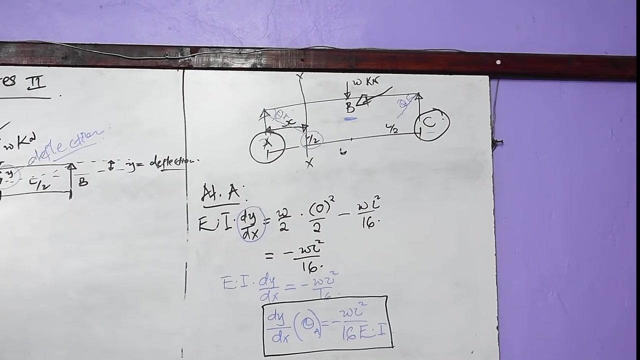 Now we want our dy over dx. Therefore, dy 1 over dx will be given by 3 wL squared 1 over 16, EI. And this is the equation for slope HC, For the deflection at point B, remember at point B we have the maximum deflection That. 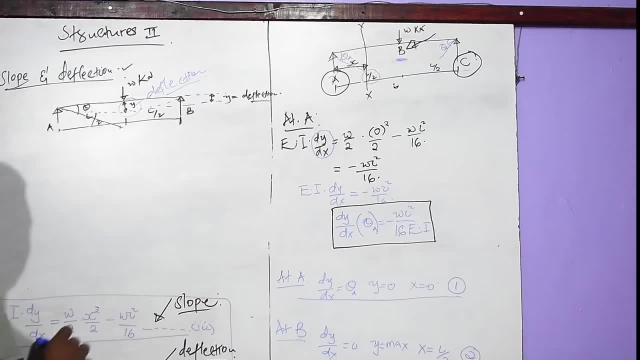 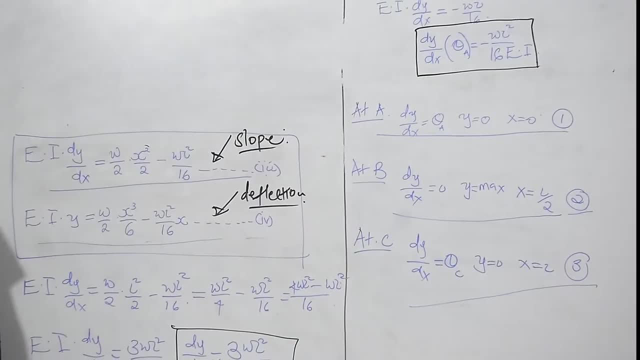 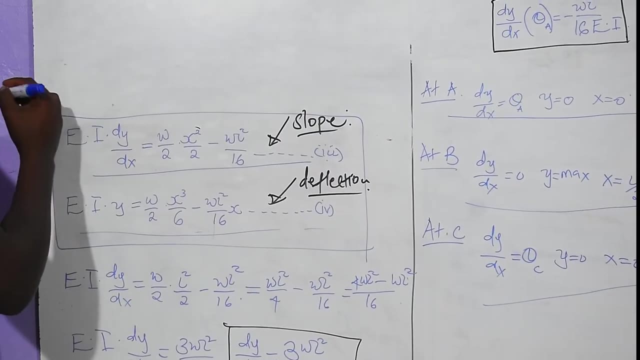 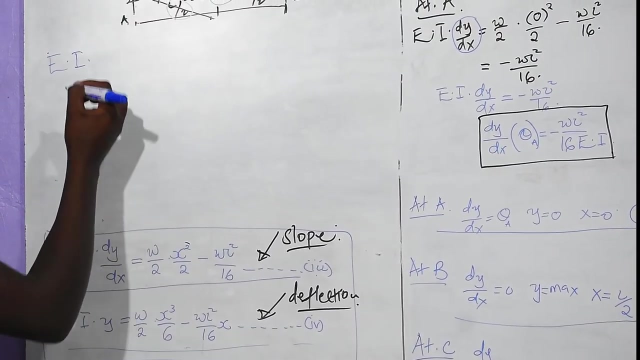 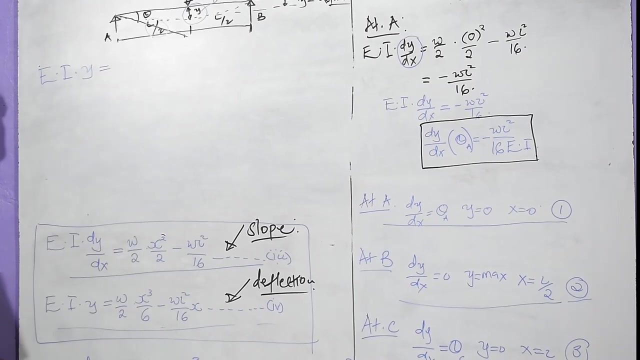 is where the beam deflects maximally. So we use the equation, equation 4, and we use the boundary condition at B. We can see in this example we have the boundary condition And the boundary condition is number 2.. Therefore we'll say EI, Y is maximum. so Y equals to w over 2, like so: 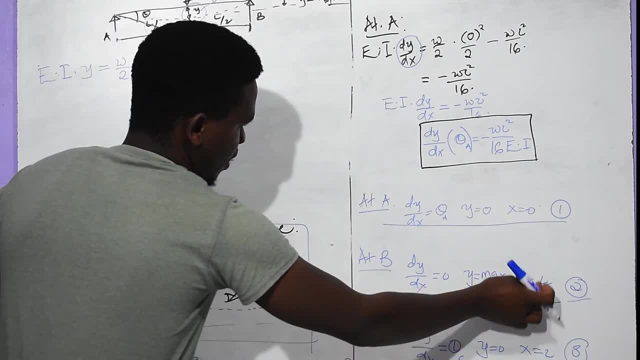 Dot x cubed. Our x is L over 2,, so l 1 over 2.. Therefore, EI dy over dx. This will be 2 wL squared 1 over 16, EI. So if you have, 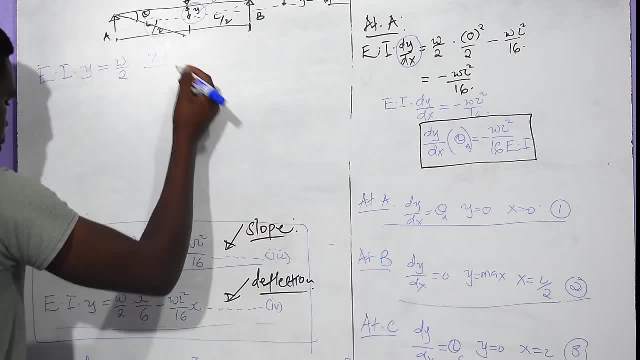 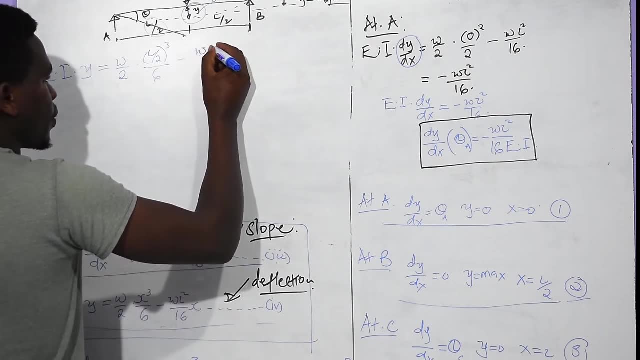 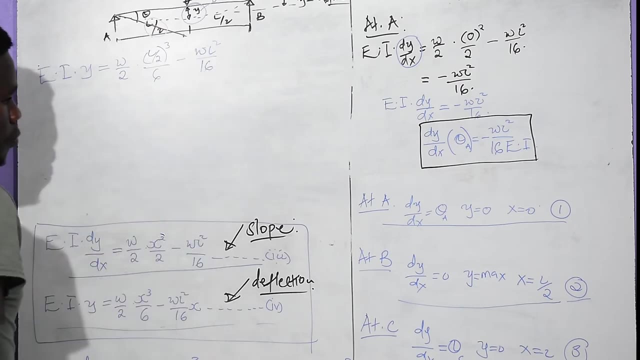 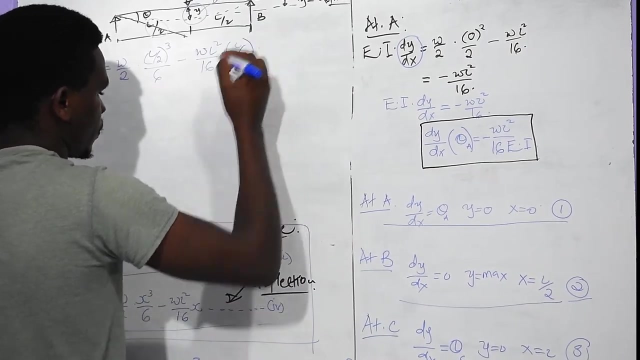 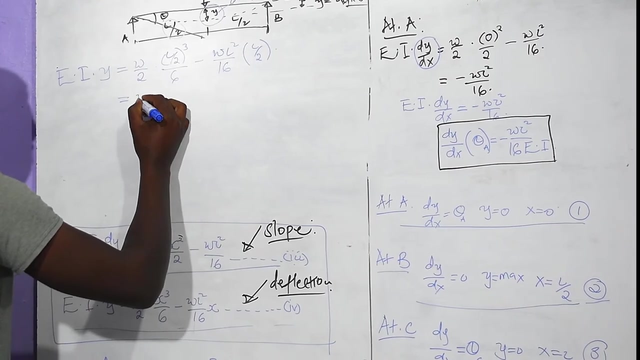 1 over 2,, cubed 1 over 6,, minus WL, squared 1 over 16, multiplied by x. But after x is L all over 2, like so. Therefore, this one will give us: this is W all over 2,. we can still combine them. 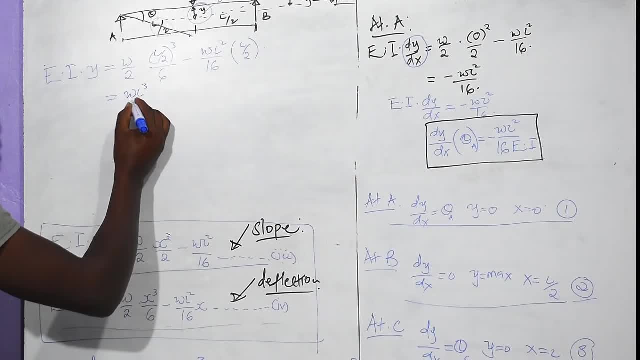 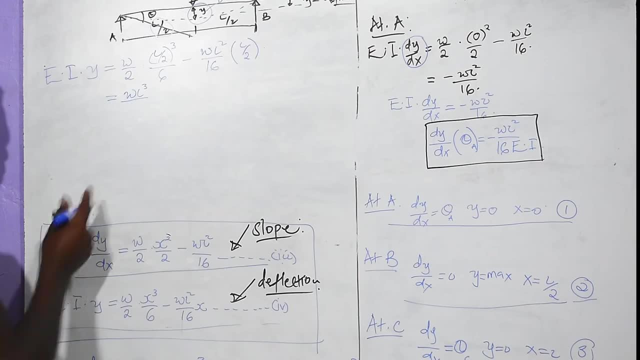 this is L cubed, so this is W L cubed all over. this is 2 cubed, that is 8, 8 multiplied by 6, that is 48, times 2, that is 96.. 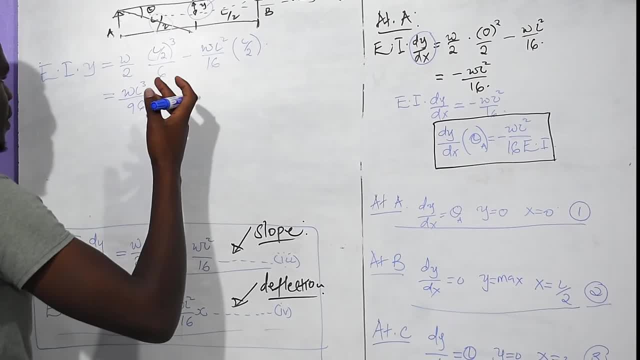 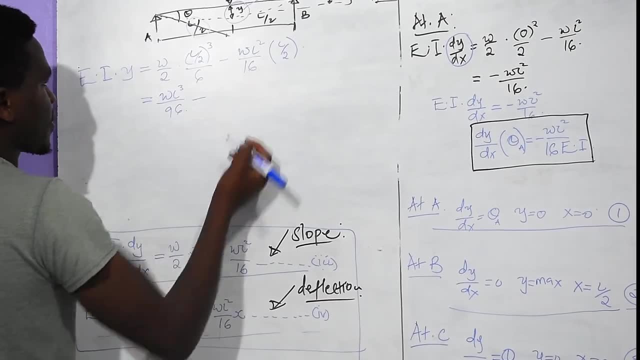 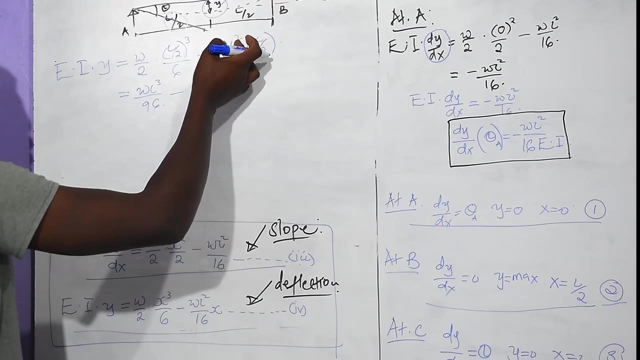 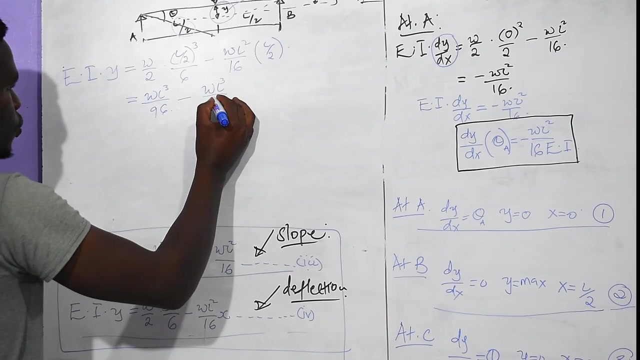 Like: so 2 cubed that is 8,. 8 multiplied by 6,, yeah, that is 96,. minus WL, this is WL squared. this is L squared. multiplied by L will give WL cubed all over. this one is 32.. 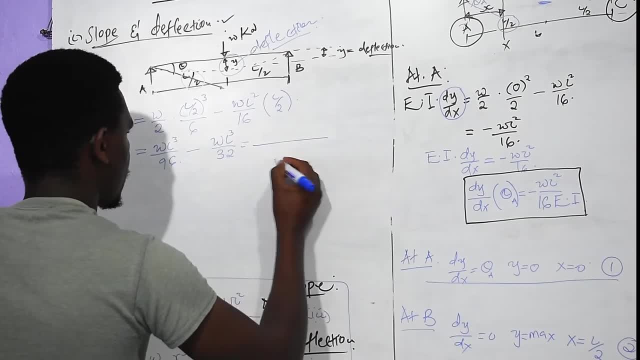 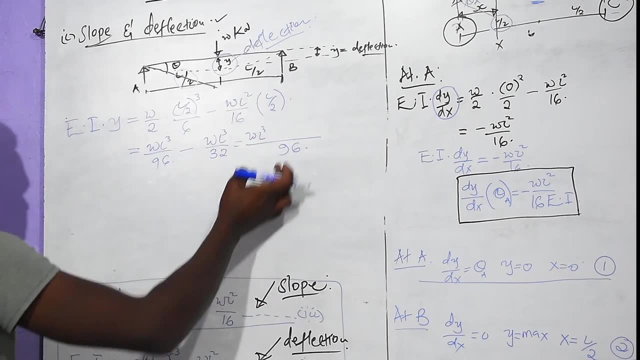 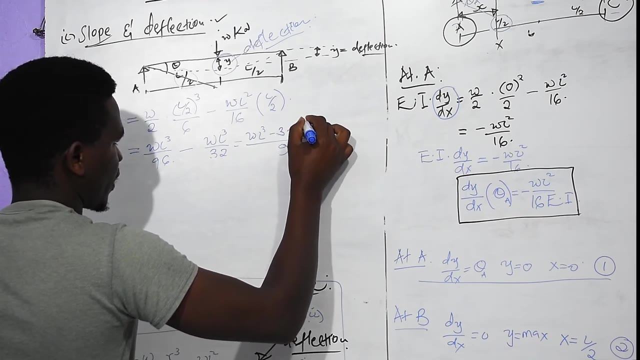 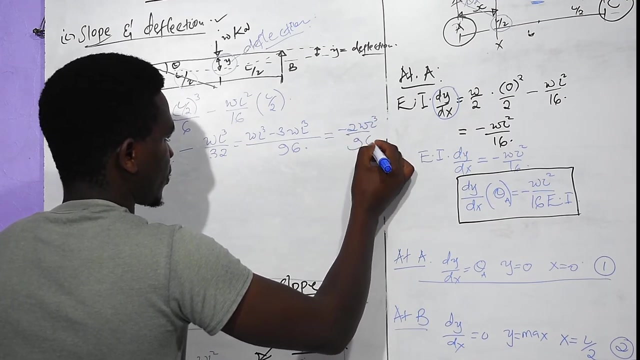 Like so. So getting the FCM of these one, This is 96, 96, so this is WL cubed 96,. you divide by 32, you get 3, so minus 3, WL cubed, you get minus 2, WL cubed, all over 96,, like so.